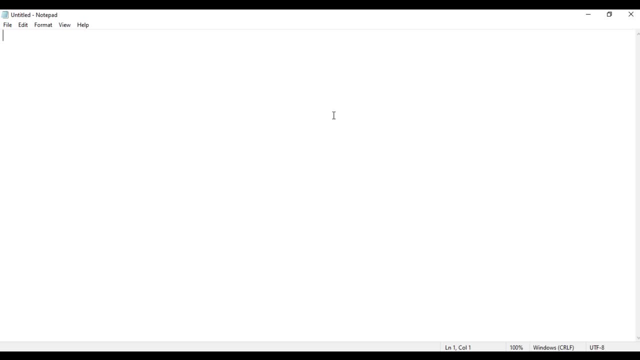 structure of any HTML5 document, I say less than exclamation. mark doc. type: HTML greater than. By reading this line of code, browsers understand the given HTML document is the HTML5 document. Our HTML document begins with opening HTML tag and ends with closing HTML tag. In the opening HTML tag I say lang equal to en. Lang equal to en indicates language of this document is: 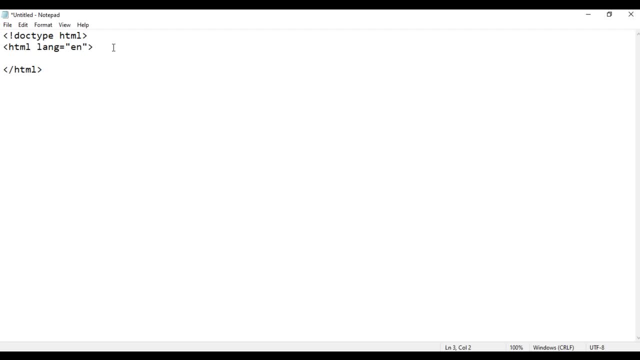 English. We know that every HTML document is divided into two sections: head section and body section. To indicate the head section, I say here: opening head tag and closing head tag. That's the head section. To indicate the body section, I say here: opening body tag, closing body tag. That indicates body section. In the head section, I say meta char set equal to utf dash eight greater than Character. 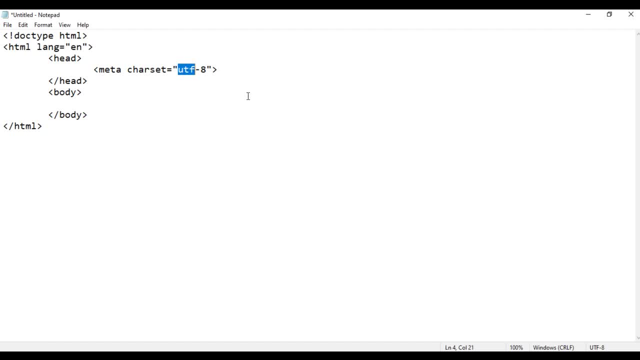 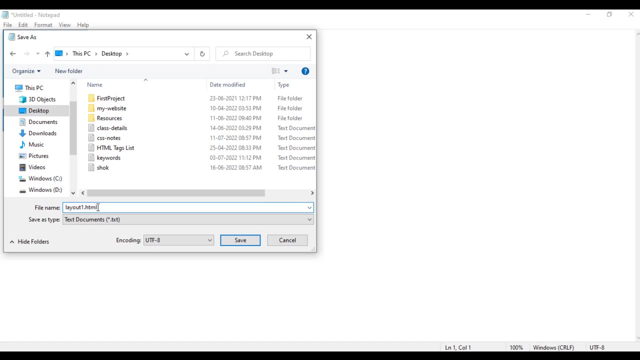 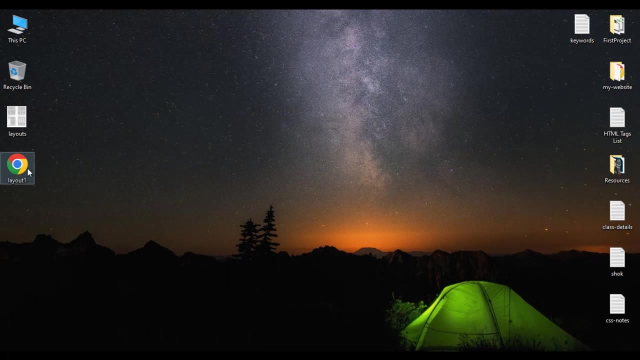 of this document is Unicode transformation format eight. That's the basic structure of any HTML5 document. guys, I'm going to save it. File save. as I save the file at the desktop with the name layout1.html, Both sides, I put double quotations and save- I minimize it. You can see that layout1.html is created. Right click, say open with. 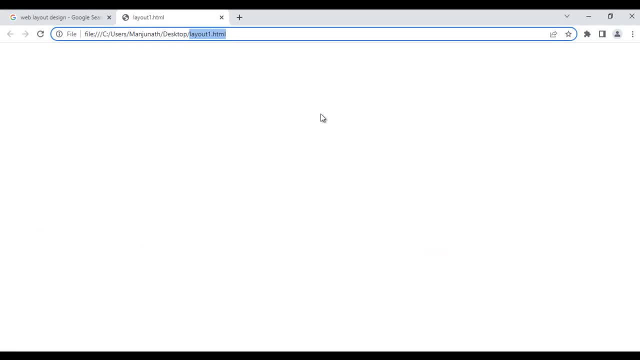 the Google Chrome You can see that layout1.html is open. in the Chrome Title is set to layout1.html, which is same as the file name. We can change the title of the web page using title tag. I say here: opening title tag, closing title tag. Inside that I say layout1.. File save. Go to browser and refresh. You can see that the title is changed to layout1. 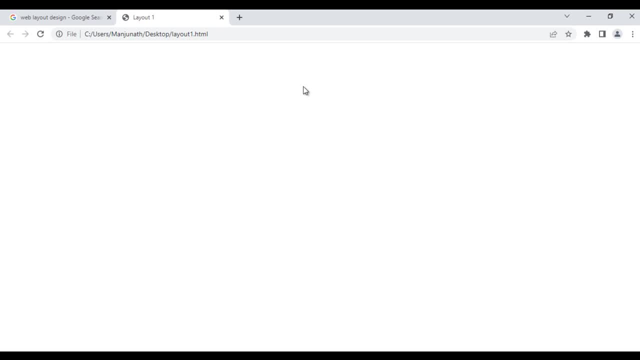 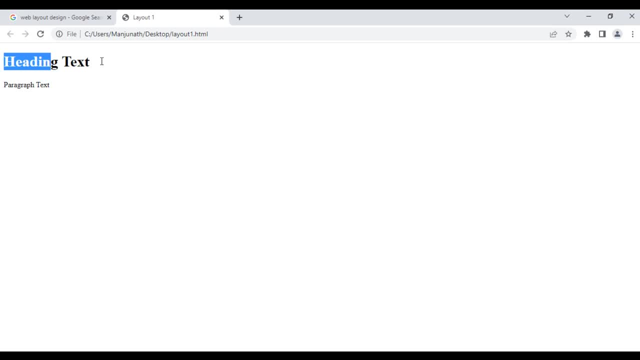 the browser and refresh, You can see that heading text is displayed, paragraph text is displayed and you can also observe above the heading text we have some space. Above the paragraph text we have some space. On the left hand side we have some space. Why? Because 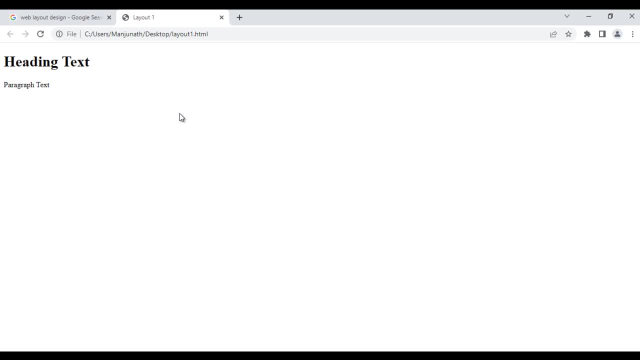 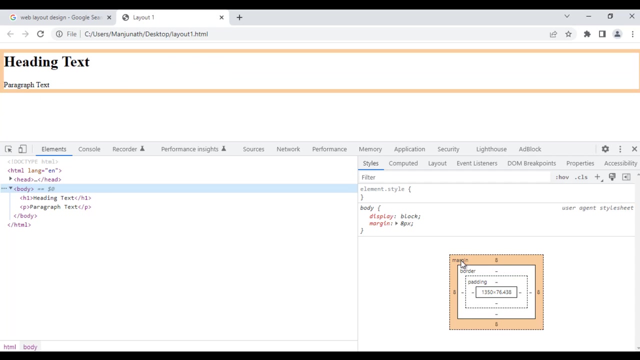 by default. some HTML elements come with margin and padding. guys, You can see here, if I go developer tools, If I click on the body tag, you can see the body tag has eight pixels margin on all four sides. This margin is applied by the browser. These are user agent styles. 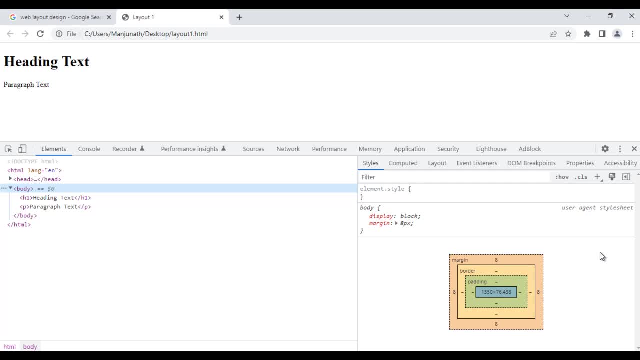 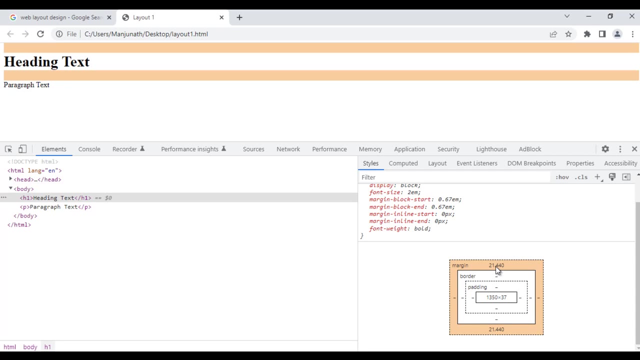 we say: guys, Okay, By default, browser applies some styles which actually called as user agent styles. So body is coming with eight pixels margin by default. If I click on H1 tag, H1 tag has 21 pixels margin at the top, 21 pixels margin at the bottom Paragraph. 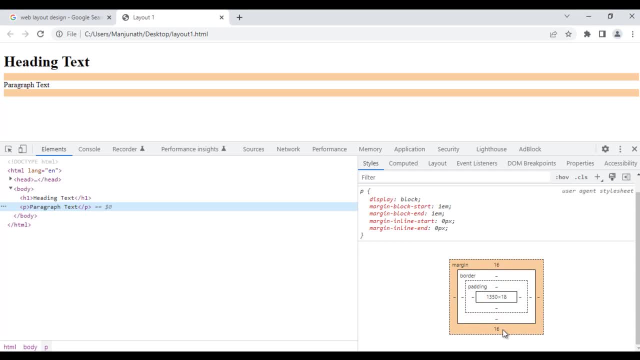 also has 16 pixels margin at the top, 16 pixels margin at the bottom. So by default, some HTML elements come with margin and padding. We don't want to have any margin and padding initially. We want to remove the margin and padding from all the HTML elements. 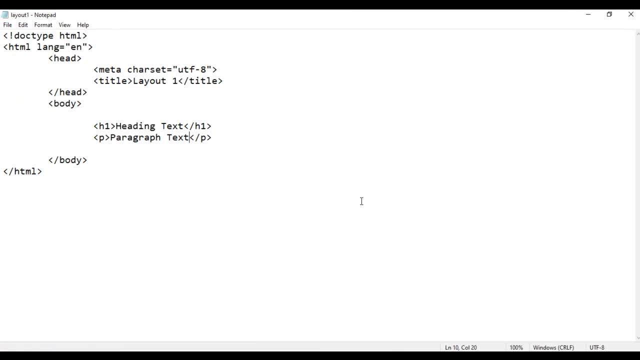 Okay, So we are going to remove the margin and padding from all the HTML elements. So that's called normalizing. So what are we going to do here? is I say opening style tag, closing style tag, and then I say type is equal to text or CSS. We are telling to the 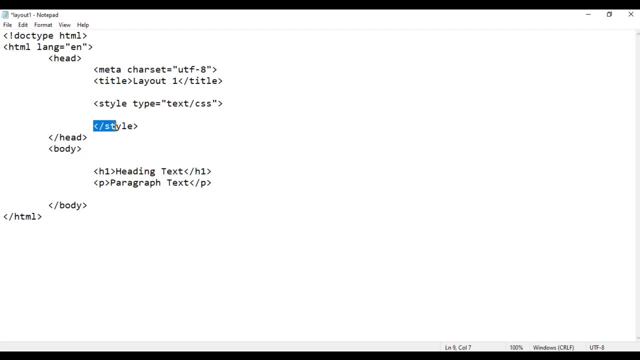 browser. anything I write in between opening style tag and closing style tag, please consider that as CSS code. Okay. And then I say here: star star indicates universal selector. We are telling: please select every HTML element in this page. Star means select every HTML. 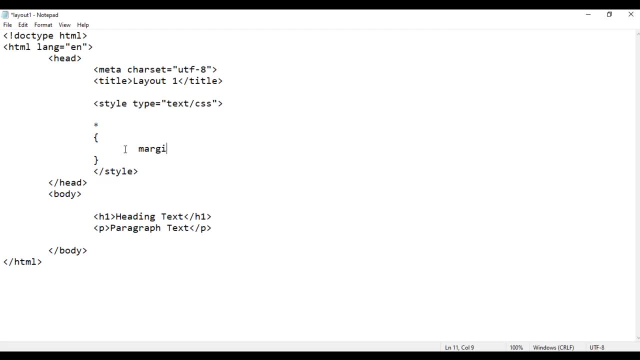 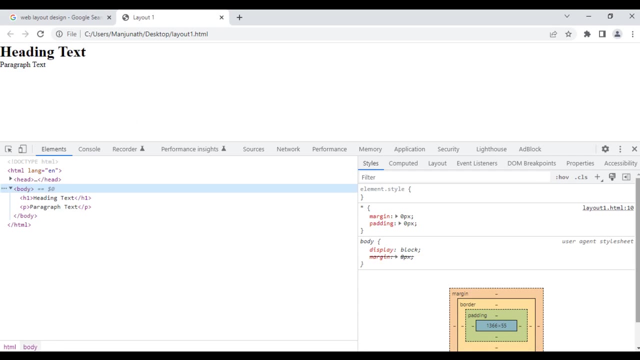 element in this page and remove the margin: zero pixels. padding: zero pixels. If I say file save, go to browser and refresh. You can see that margin is removed from all the elements. Margin is removed from the body. You see, body has no margin. H1 also has no. 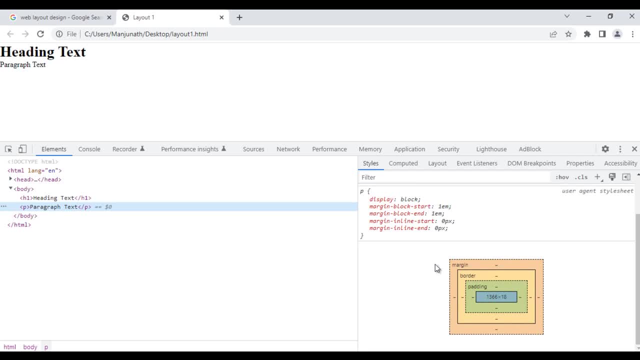 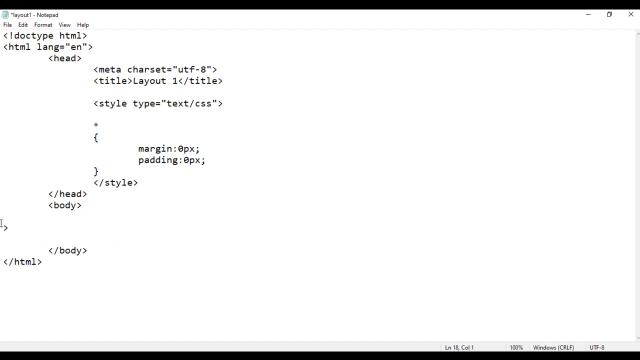 margin is removed from h1 also. margin is removed from the paragraph also. so that's what the star does. star selects every html element. guys, i hope it's clear to you. good, now we understood what is the meaning of normalizing. next we are going to understand the box sizing property, which is: 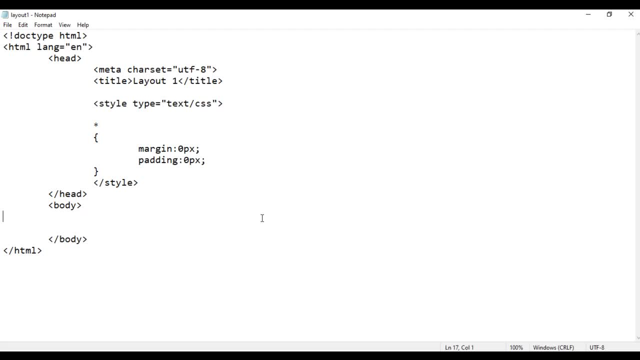 again very important to understand. i say ctrl s to save. here i am going to say opening to closing div. inside that i write the text do one and i'm going to identify it uniquely by giving an id of due one. if i say file save, go to browser and refresh. you see, do one text is displayed next. 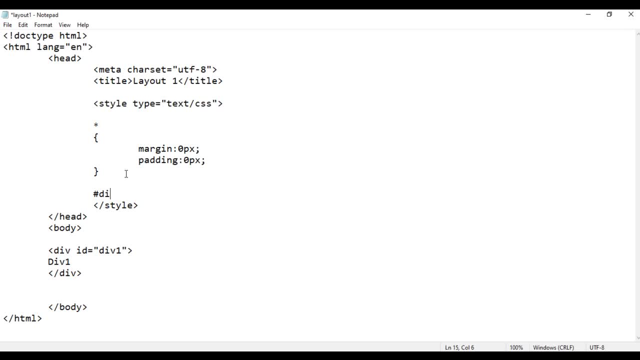 i am going to apply some styles here. i say hash due one, opening flower bracket, closing flower bracket. so i am telling: select any html element which has the id attribute value set to due one. so this html element id attribute value value is due1.. Its width should be 100%, So it should occupy the entire width of the browser. 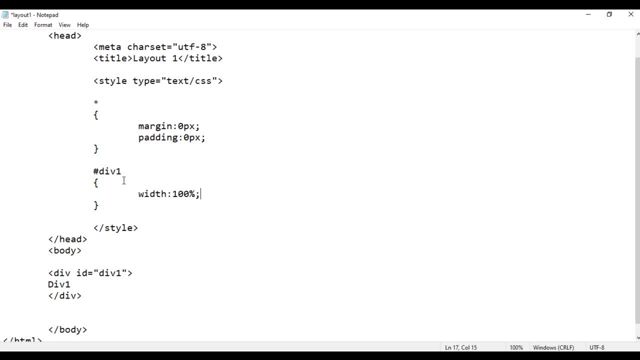 Its width should be 100% of the parent. Parent is the body type, Okay, next, HEIGHD: Height should be 50 pixels and then background-color should be light gray. If I say file save, go to browser and refresh. You can see that our due1 has width: 100%, height, 50 pixels. 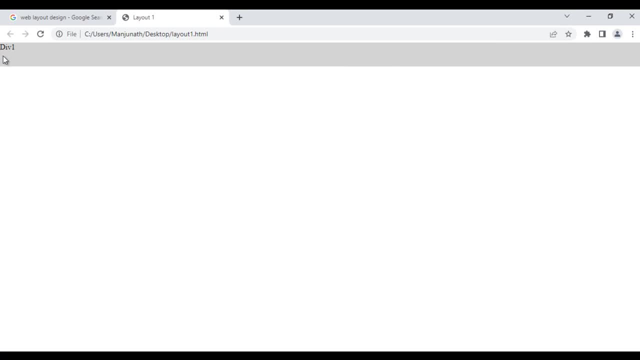 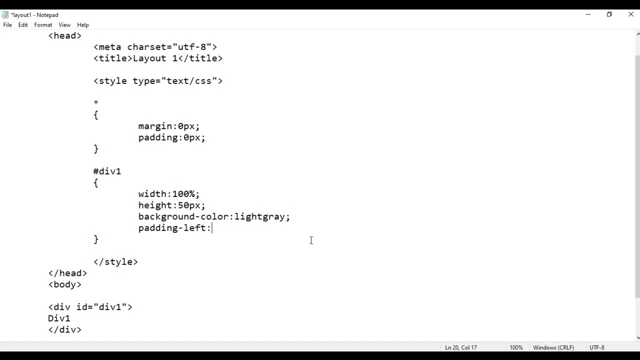 background-color: light gray. Good, Now I want to add some padding on the left side and right side. So if I come here and say p-a-d-d-i-n-g padding-left 2% padding, I want to add Similarly padding-right- 2%. If I do like this, check out what happens If I say file save go. 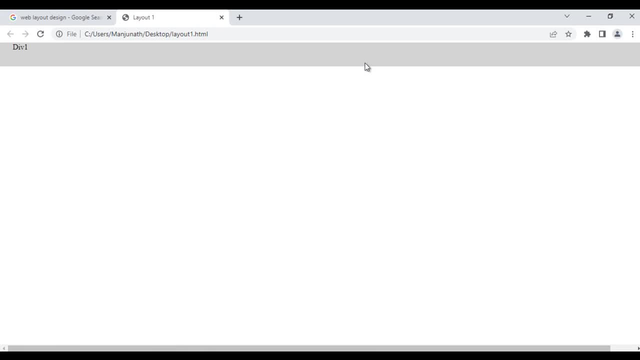 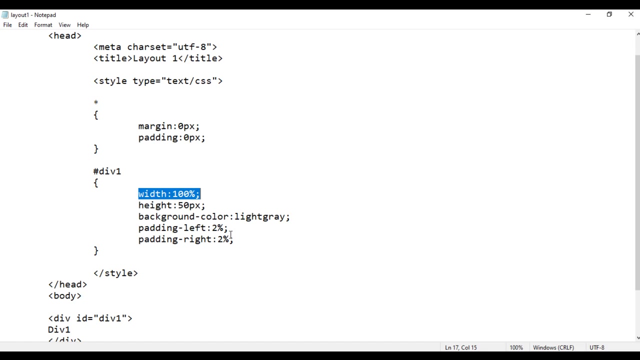 to browser and refresh. Our due1 is going outside the browser now. You see, we are getting the scroll bar right. Our due is going outside the browser here. Why? Because the width of this due 1 is now 104%. guys. The actual width of the due is calculated like this: Weak plus. 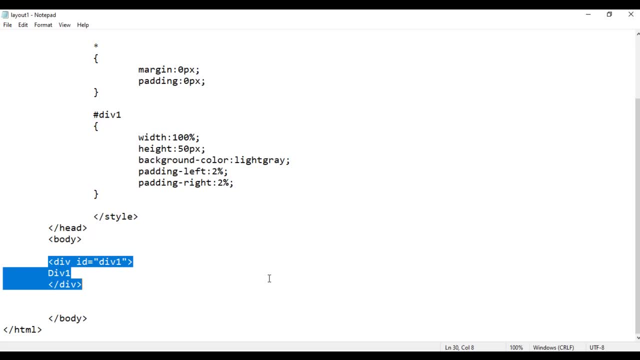 padding left plus padding right, Plus padding one more time. Save, Go to browser and refresh. cute, I did it already. It's my test. Save, go to browser. Save, Go to browser and refresh. Our dude is going outside the browser now. You see, we are getting. 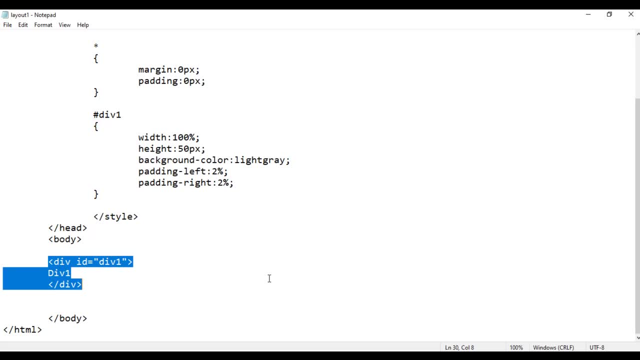 border left plus border right, plus margin left plus margin right. guys, That's the actual width here. Here, the actual width of this div 1 is 100%, padding left, padding right: 4%, So total 104%. If I have to make this div 1 100% only, then what I have to do, I have to subtract 4% from. 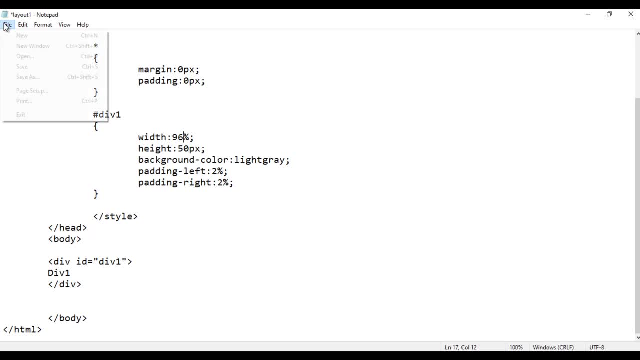 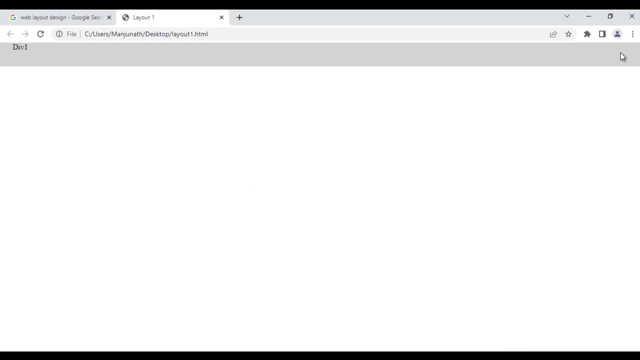 here. If I say 96%, file save, go to browser and refresh. You see the scroll bar is gone. Our div now has exactly 100% width, It's not 104%. Okay, good, If I come here and remove the padding, if I remove the padding from both sides, if I. 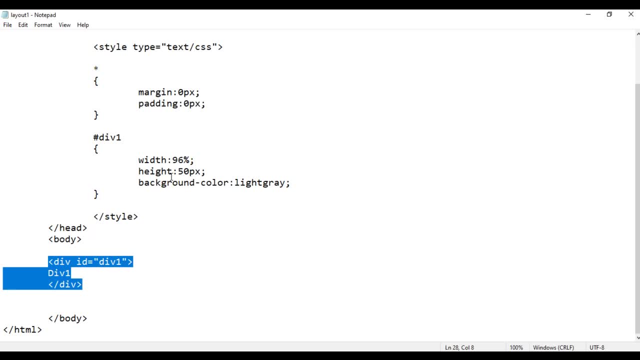 say save. now. the actual width of this div is 96%. If I come here and refresh, you see it has 96%, Not 100%. To make it 100%, of course, I have to add 4% here. I say 100% now file save. go to browser and refresh. 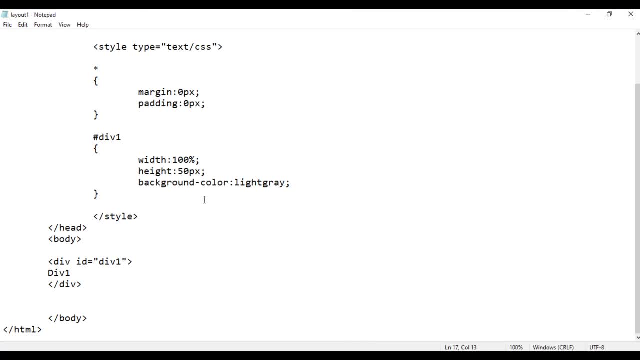 Now it is 100% right. So whenever we add padding or border, we have to change the width value. Either we have to add or subtract. To remove this disadvantage of adding and removing the value to the width, we have an option called as box sizing. 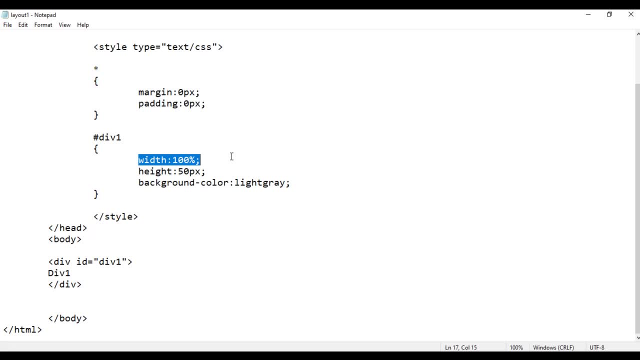 We have a CSS property called as box sizing guys. So if I come here and say box sizing, border, dash, box, When we use this CSS property you can add padding and border without worrying guys. You need not worry about adding or subtracting the value from the width guys. 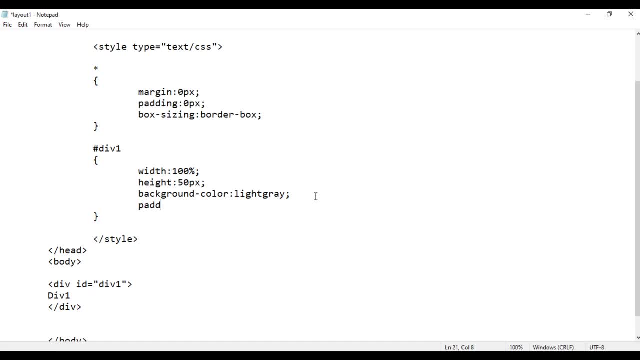 So if I come here and say PAWDING- Okay, PAWDING padding dash left, 2%. and if I say here, PAWDING padding dash right, 2%, Now the actual width of this div 1 is still considered as 100%. 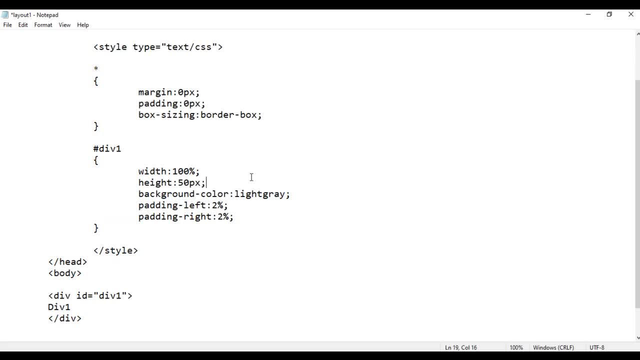 Padding left and padding right are now the part of the width guys, So you need not to worry about subtracting here, You need not to make it 96%, Just say file save, go to browser. go to browser and refresh, You see. 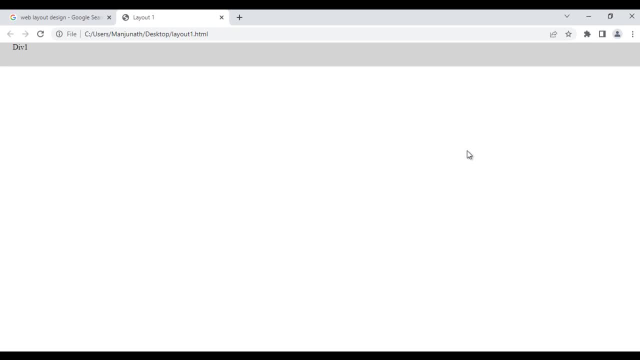 We have the padding added and our div is not going outside the browser. So when you add padding or border, it is considered as part of the width guys. You need not to do any modification to the width. The width is still a hundred percent only. 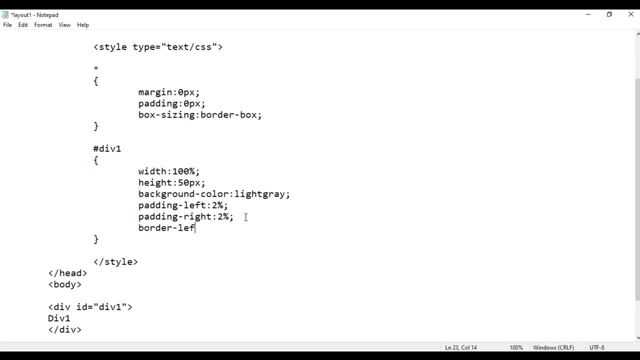 So if I say here, for example, if I say border dash left, border left, let's say 20 pixels solid black color. Similarly, Border Dash White, 20 pixels Solid Black. If I say file save, go to browser and refresh. 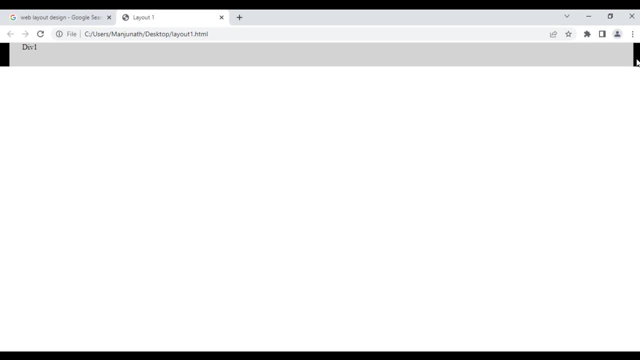 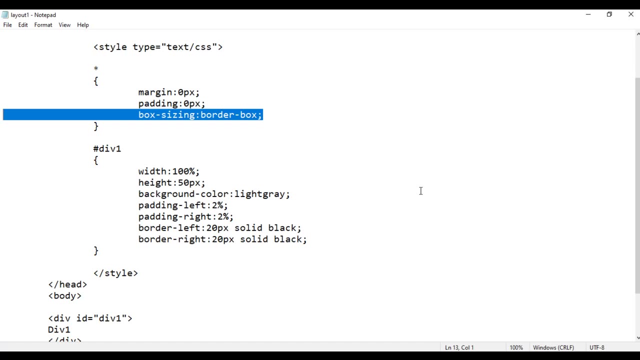 You can see the left right side. we have the border 20, 20 pixels. Our div width is not changing. It is not going outside the browser. If this box- sizing border box- is not available, if I say control X and save, come here and 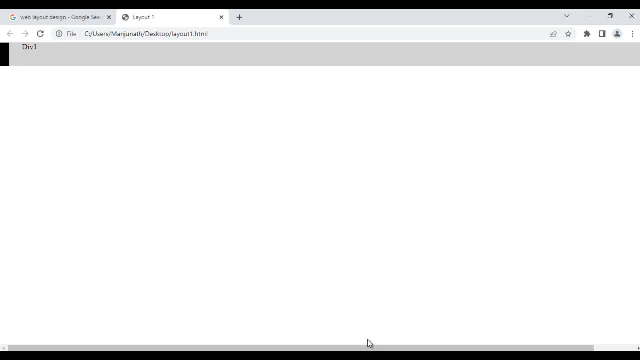 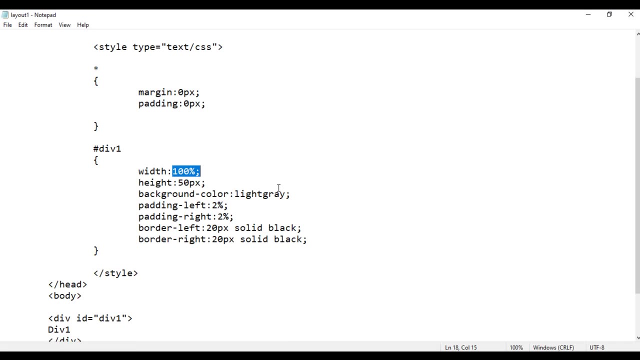 refresh. definitely the div goes outside. guys, You see that it's going outside, So you have to Subtract the width value, all that thing you need to do. So that problem is solved with the help of this box sizing, border box. So, box sizing, border box: save. go to browser and refresh. 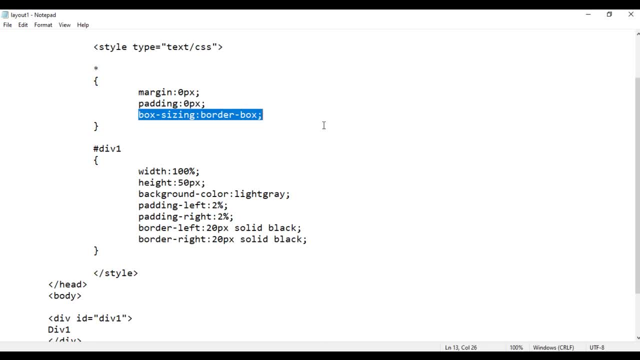 So when do you use box sizing, border box? You are just telling that please consider padding and border as part of the width to the browser. You are telling that, So now you can easily add padding and border without worrying of adding or subtracting. 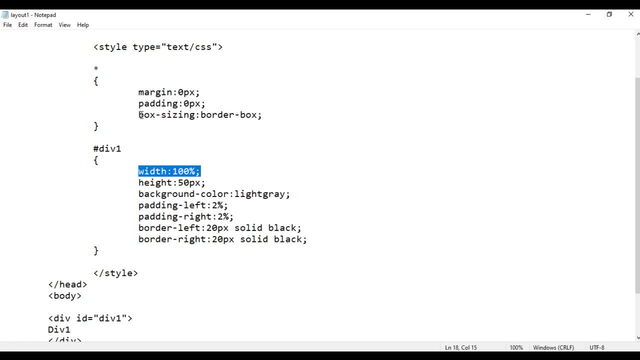 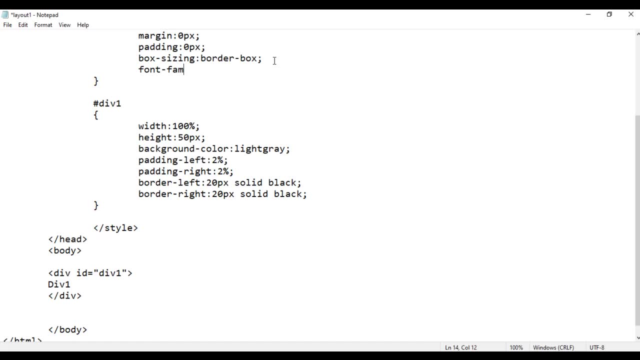 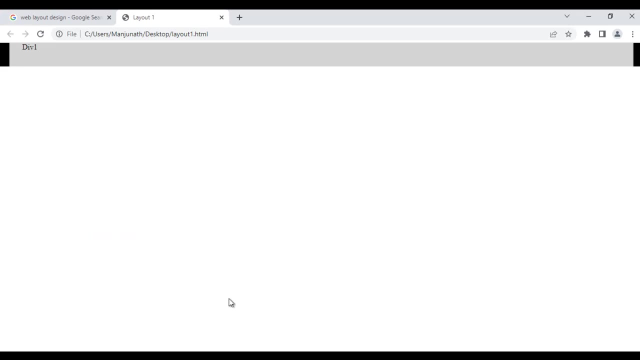 The value from the width. Simple thing, Good. So that's about box sizing, border box- Good. Next I'm going to set the default font. I say here: font family of of Arial. semicolon file. save. go to browser and refresh. 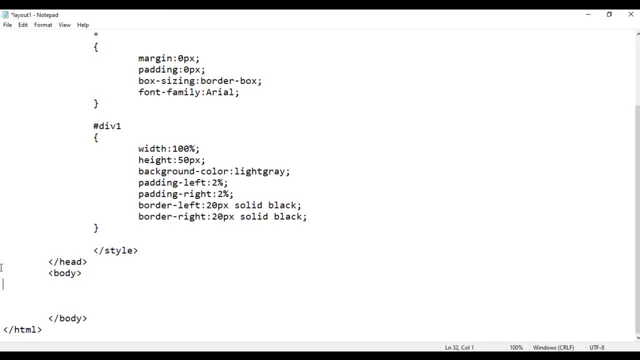 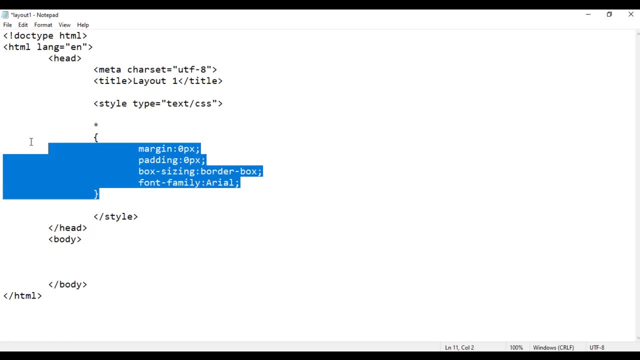 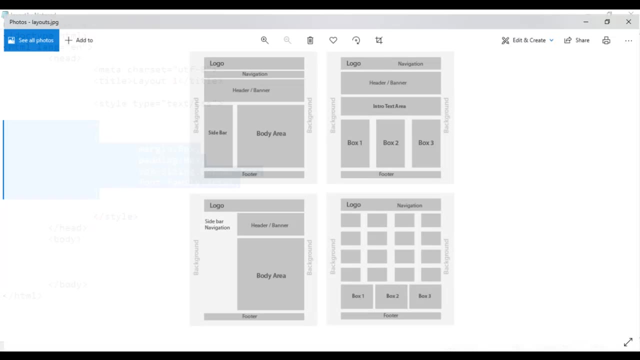 So Arial font. Now we understood the necessary CSS properties for normalizing the page, right? So? So this code we write in every web page, guys. Okay, File Save. Now let's begin designing the layout. So first we are going to create this div, guys. 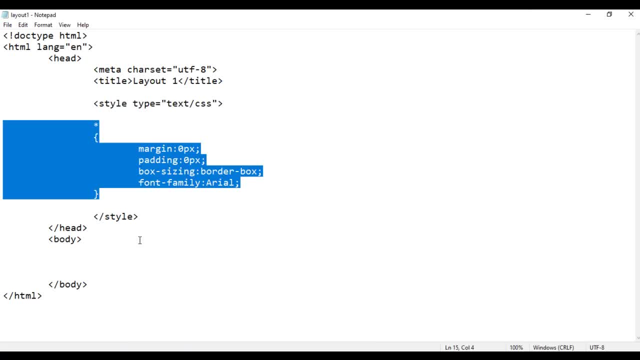 So let's start with this div. Okay, We're going to create first div. So I say here: opening div, closing div, I'm going to give ID to it as logo dash div and inside that I put the content logo. If I say file save, go to browser and refresh. you see, the logo text is displayed. 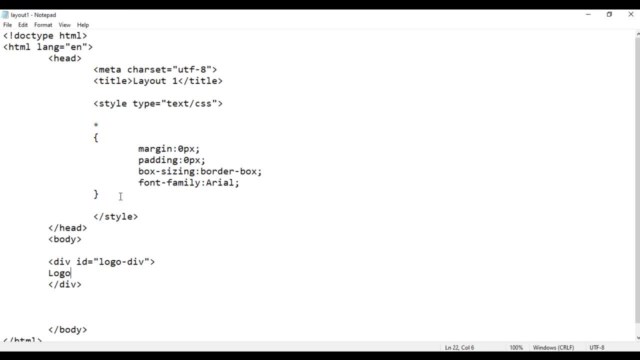 Good, Let's apply the CSS styles. To apply the CSS styles, I say here: hash LOGO logo. div. opening, closing flower bracket Width should be 100%, Height should be. we can use instead of height minimum height: H E, I, H E, I, G H T. 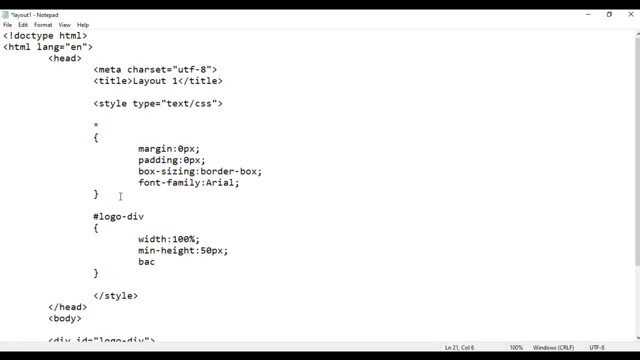 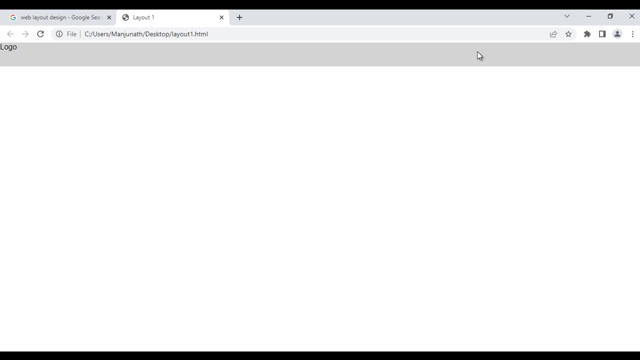 Minimum height Should be 50 pixels and then background dash color should be light gray. If I say file save, go to browser and refresh. You see we have our div with the width, 100% height, 50 pixels and background color light. 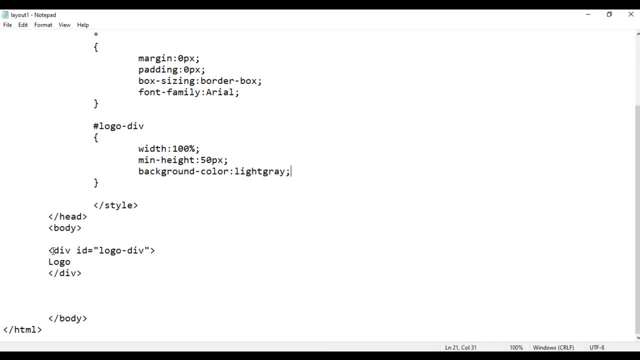 gray right. So whenever you are designing a section, first you set these three properties. go and see in the browser what is happening. That gives you an idea Of what to do next. Okay Now, what to do next Next? you can see here: we want little bit left padding for the logo text, right. 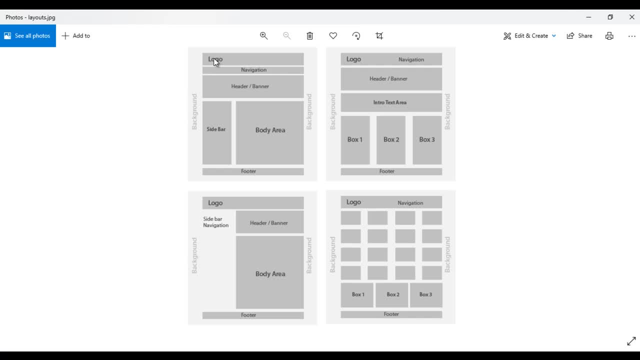 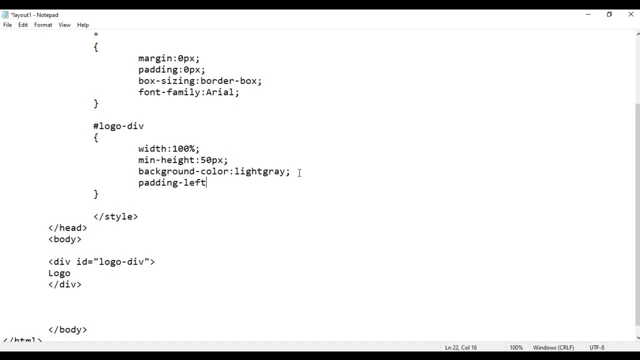 You can see there is a padding we have on the left side. here Logo text is a little bit inside right. So for that, what are you going to do? You are going to say here: P A, double D, I N G padding, dash left of 2%. 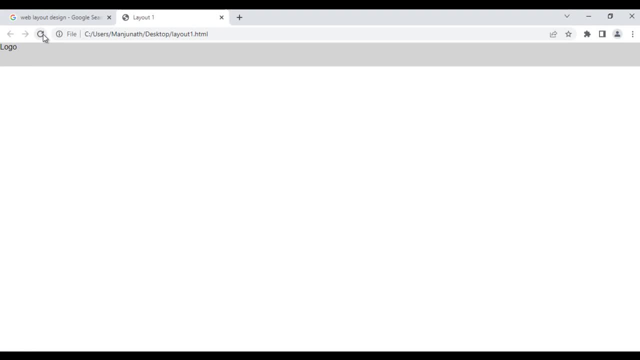 If I say file save, go to browser and refresh. You can see the padding left is added. I want the logo should be vertically centered. For vertically centered what we have to do, we have to increase the height of this line, guys. 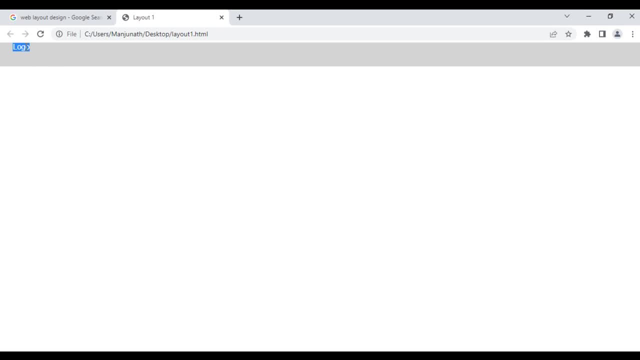 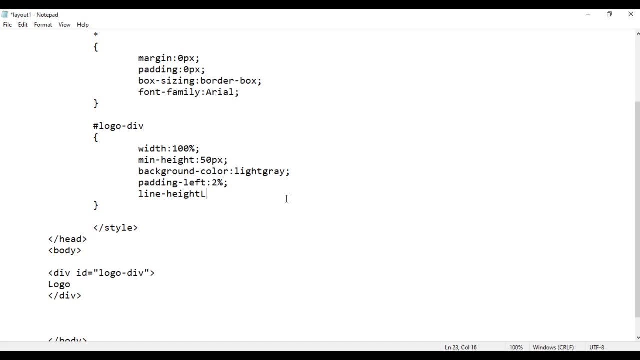 We have to increase the line height of this logo text. So this blue box indicates the height of the text here. So, simply, what I do, I say here: L I N E line dash height. Line height should be same as the minimum height, what we are setting here, which is: 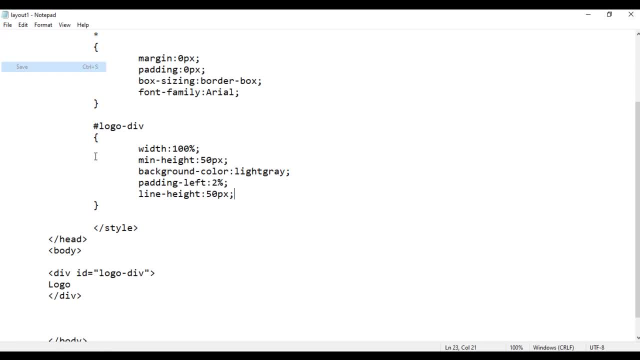 50 pixels. If I say file save, go to browser and refresh. I want the logo should be vertically centered. For vertically centered what we have to do: Go to browser and refresh. You can see that the logo text is vertically center line. 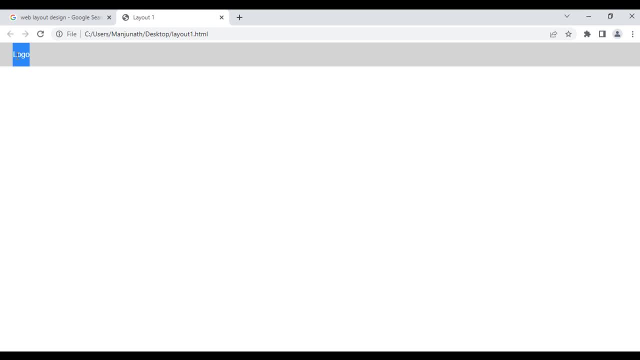 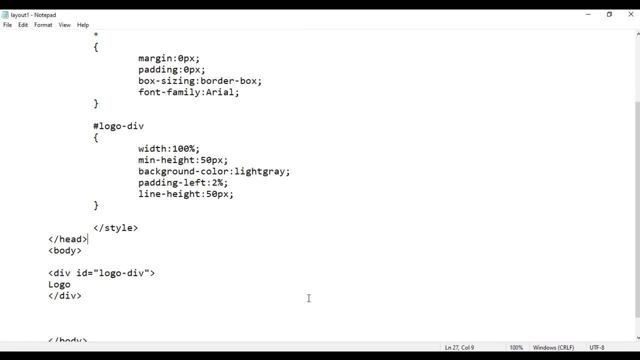 So if I select this, you can see height is increased. Always the text is displayed at the center guys of the line. Okay, So that's what you do. We are successfully able to create the first div. Let's create this below: div navigation div. 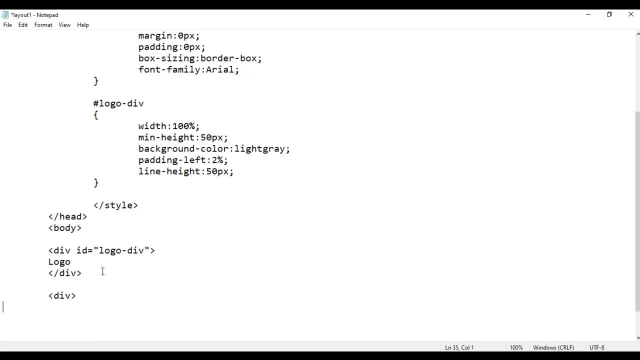 So what we have to do below this div, we are going to create one more div- opening div, closing div- and the text we display: navigation, Okay, Navigation. And I'm going to set the ID here. ID of nav dash div. 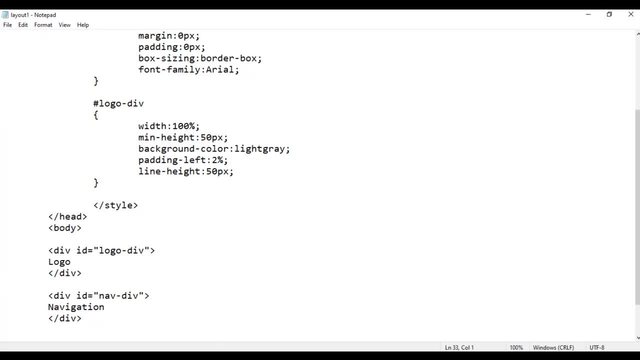 That's our HTML code file, save. go to browser and refresh, So navigation text is displayed. Let's apply the styles. So to apply the styles, what we do, we say hash nav, div. opening flower bracket. closing flower bracket. 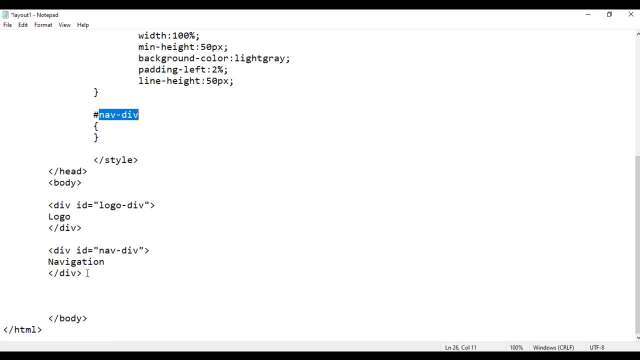 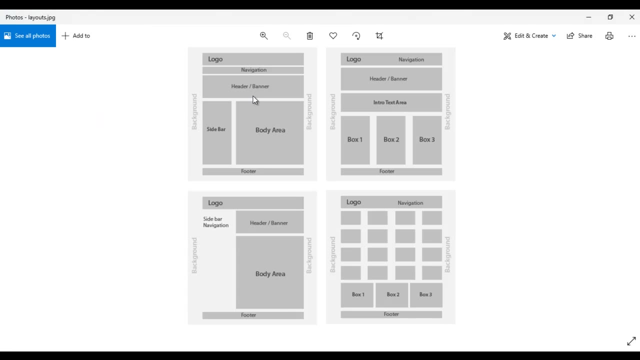 We are telling: select the HTML element with the ID nav div. This HTML element has the ID nav div. Okay, It's style should be: width should be 100% and the minimum dash height should be 30 pixels. You can see that this div has less height. 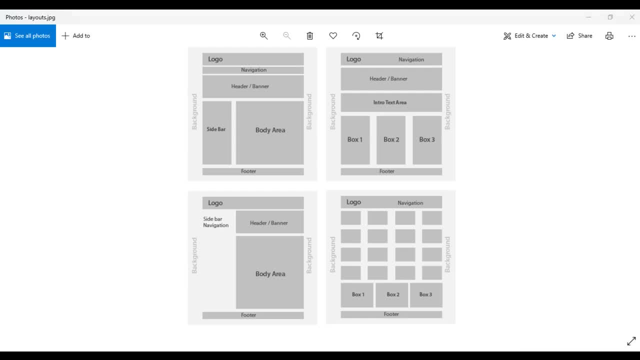 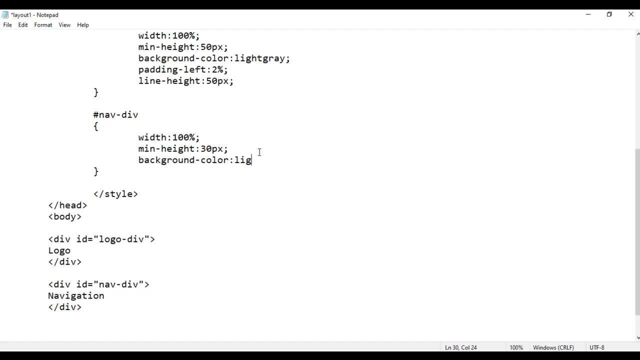 Navigation div has less height than the logo div right, So 30 pixels I'm setting here And then B-A-C-K-G-R-O. even the background dash color should be L-I-G-H-T- light gray. Okay, Let's go to the properties. 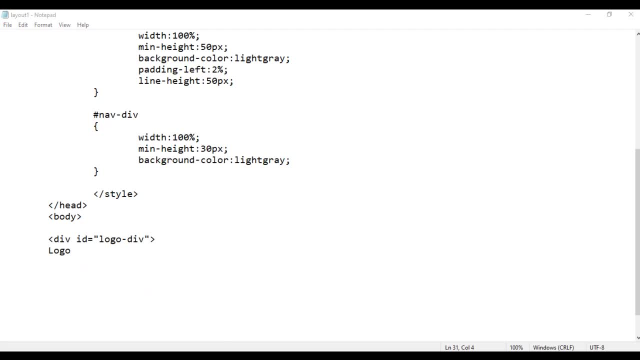 Go and check what is happening in the browser File, save, go to browser and refresh. Okay, We got it, But we need some gap in between the logo div and navigation div. right, You can see here we have some space here. 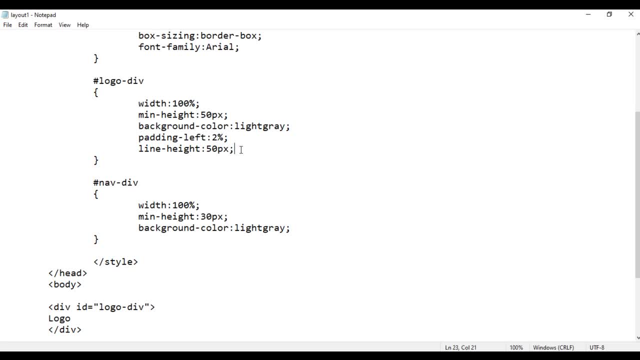 For that. we are going to add margin bottom to logo div. So here I say M-A-R-G-I-N- margin dash bottom of 10 pixels. If I say file save, go to browser and refresh. You see, We got some space here. 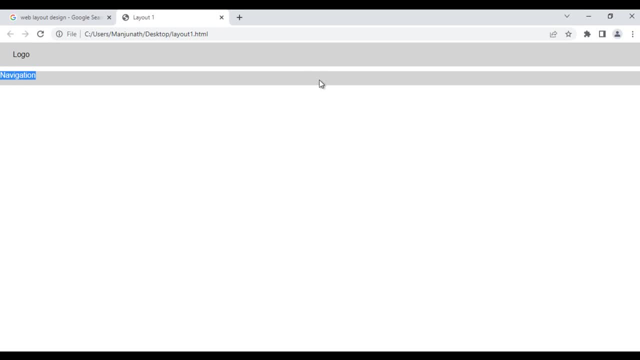 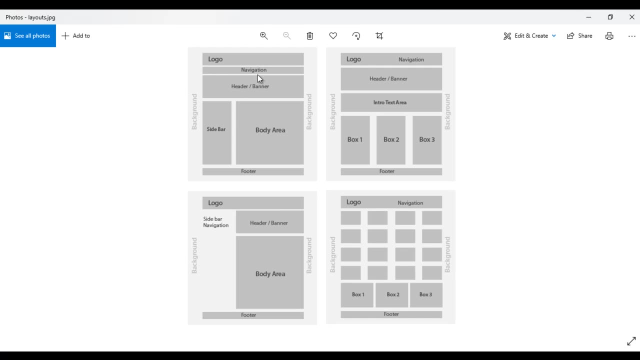 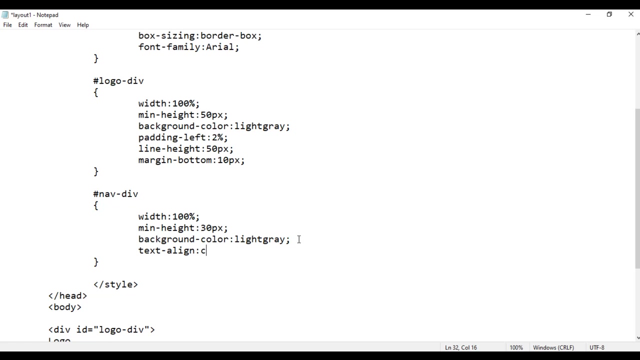 Good. Next we have to place this navigation text in the center align. You can see here navigation text is center aligned horizontally and vertically. For horizontally center aligning the text we use text align property text dash align center. I say file save. go to browser and refresh. 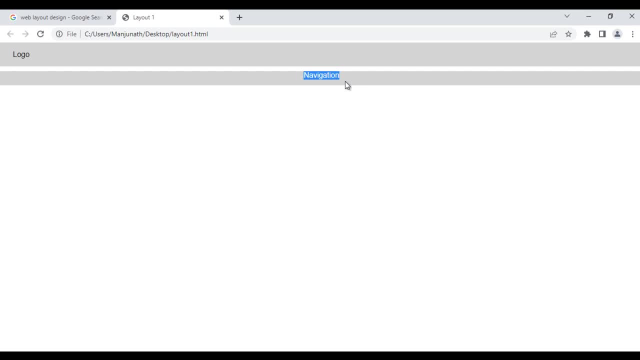 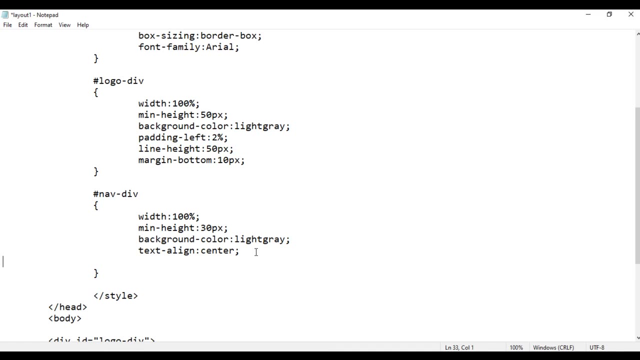 You can see, the navigation text is horizontally center aligned, not vertically. So vertically center aligned. what we have to do, We have to take help of the line height property. So here I say L-I-N-E, line dash height, which should be same as the minimum height of the 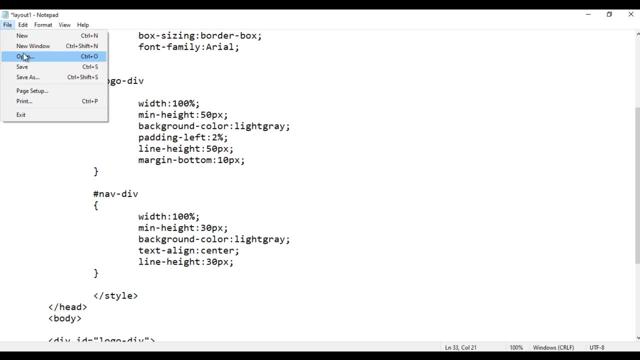 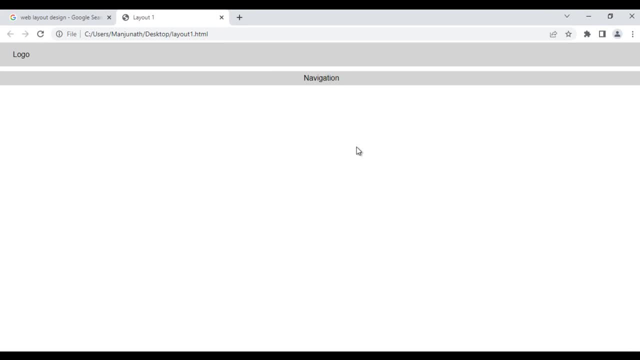 div. So I say here 30 pixels. If I say file save, go to browser and refresh, you can see that navigation text is vertically center aligned. Very simple, right? That's how you design the layout step by step. Okay. 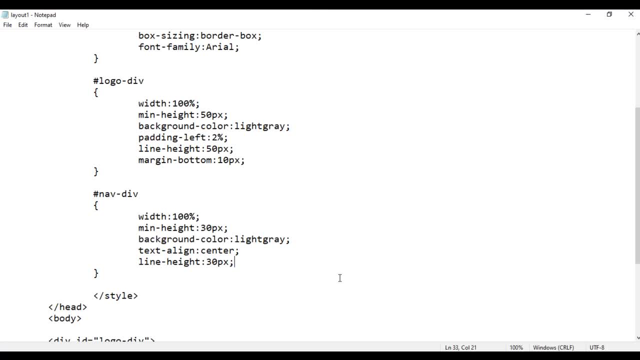 Next what we have? Next we have header banner div. Very simple, I come down here. I create another div: opening div, closing div, The text we display here: header forward, slash banner and ID. I am going to set here H-E-A-D-R. 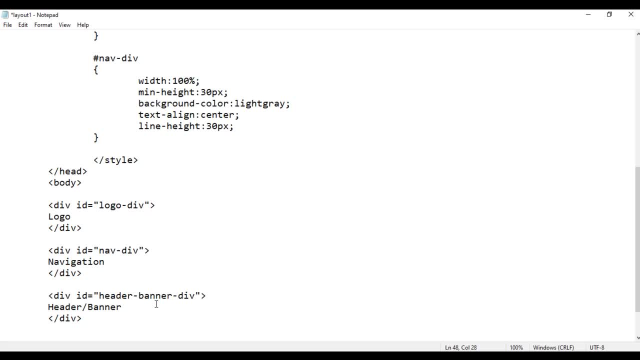 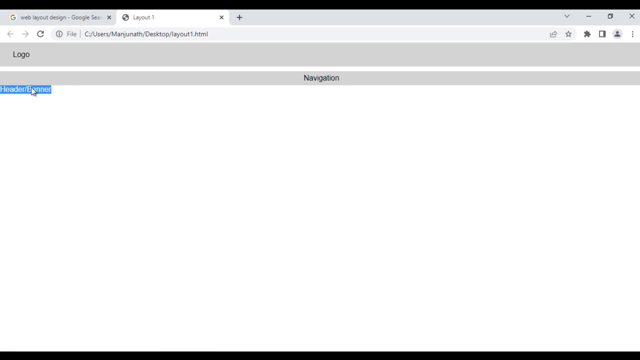 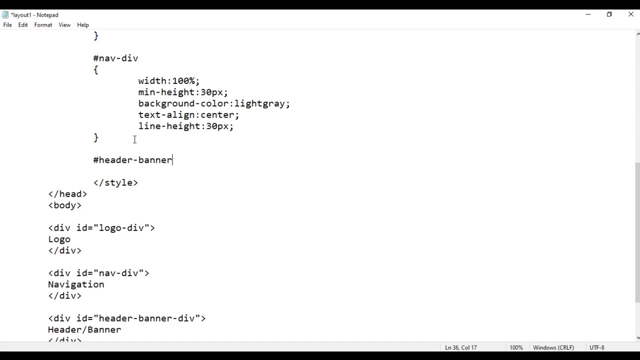 header banner- dash div. Okay, I say file save. go to browser and refresh. Header banner text is displayed. Let's apply the styles. So here I simply say: hash- H-E-A-D-R banner- dash div. H-E-A-D-R. header banner- div. opening- closing flower bracket. 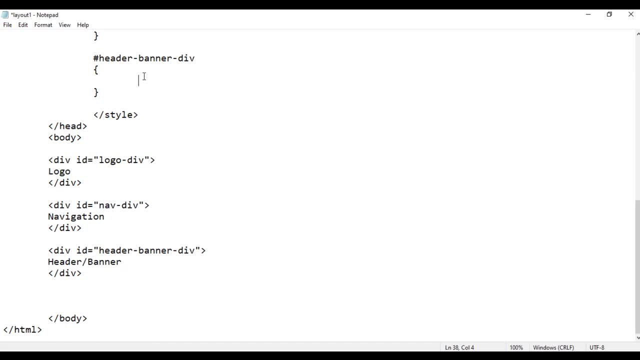 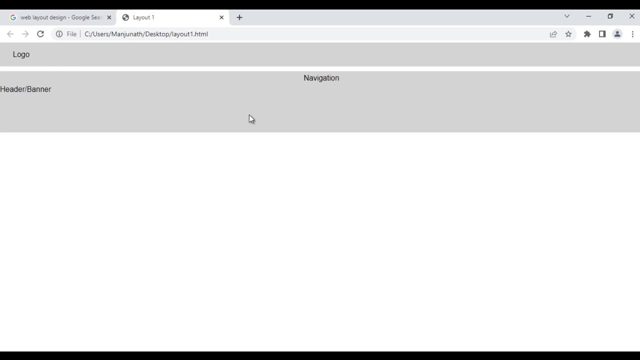 Okay, Now let's apply the styles I say here. width should be 100% and then minimum dash height should be 100 pixels. background dash color should be light gray file save. go to browser and refresh. You can see that header banner div is created with the styles. 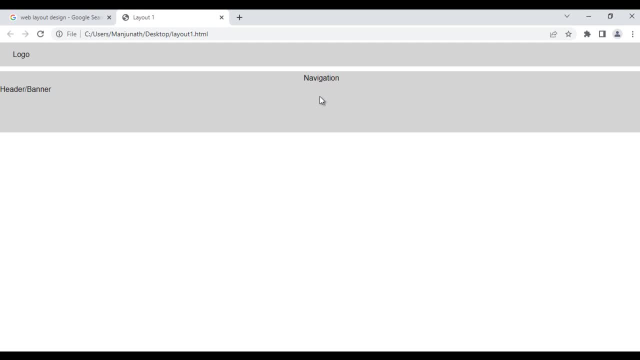 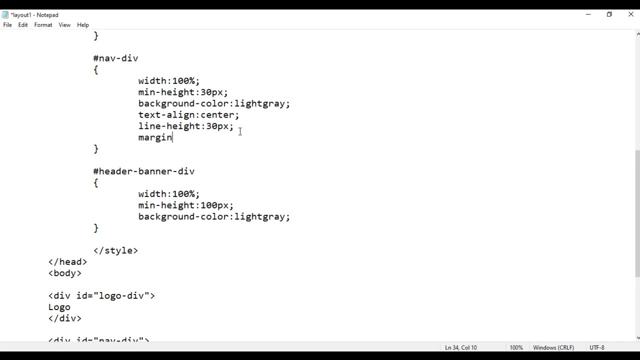 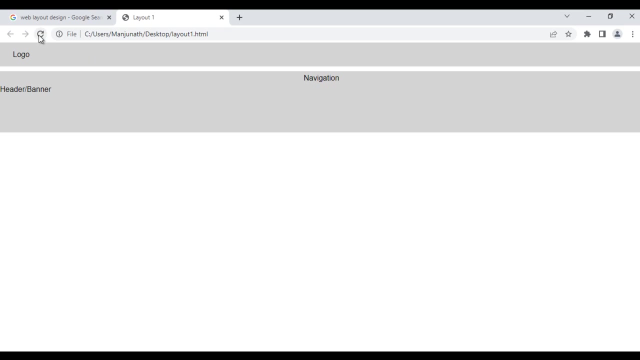 Now we need some space below the navigation text, Right Navigation div. So what we do? We go to nav div and say here: M-A-R-G-N- margin dash bottom of 10 pixels. File save. go to browser and refresh. 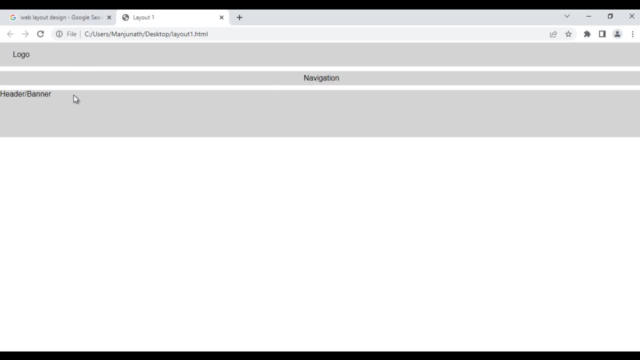 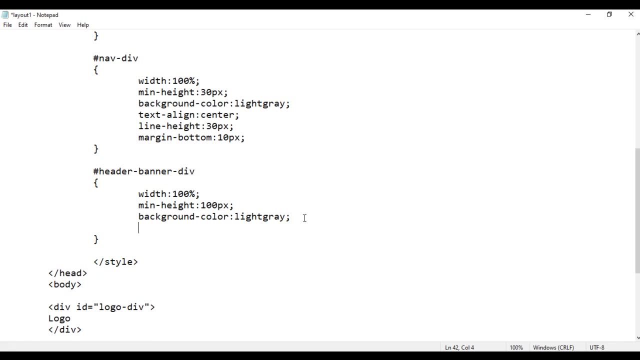 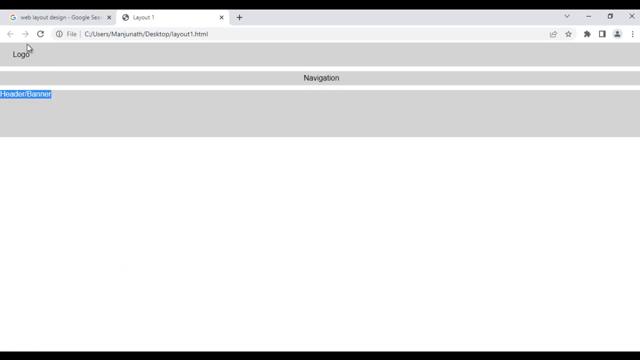 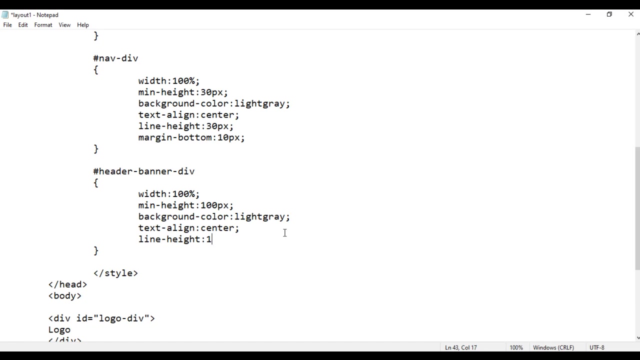 You see we got the gap. Next we have to put this header banner text horizontally center, vertically center. So h-e-a-d-r banner dash. div. for horizontally center we say text dash align center. file save. go to browser and refresh. vertically center. we take help of line dash height of 100 pixels, same as minimum height. 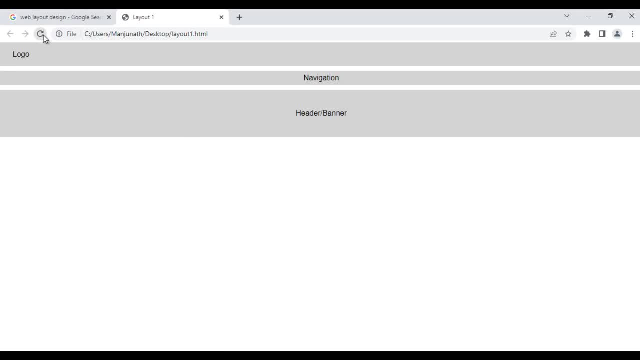 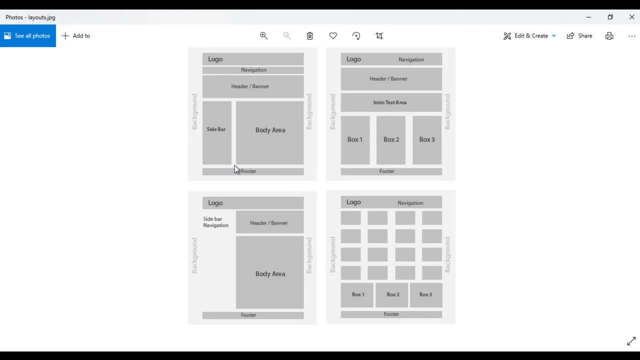 file save. go to browser and refresh. see header. banner text is displayed in the center: guys, very good. next we are going to display a sidebar: due and the body area do one beside another. so whenever you see the dues placed one beside another, you have to use a simple technique. 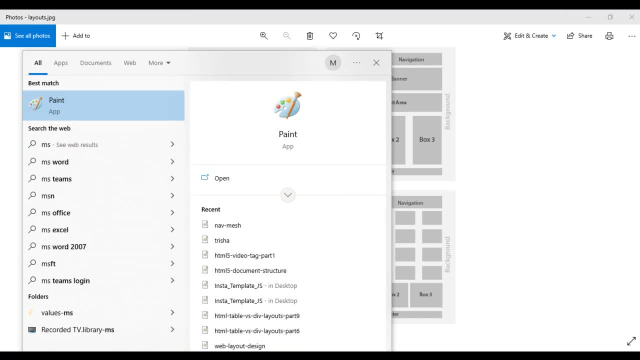 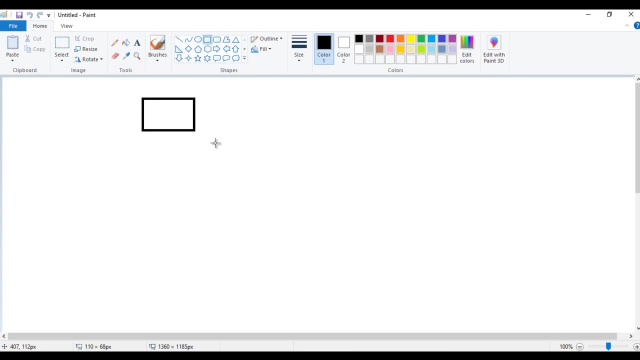 here. let me explain that. I see here, Ms paint. okay, so whenever you need to place the duos one beside another, what you do is you create one parent due, okay, and then you have to create the children's the dues which should be placed one beside another. they should: 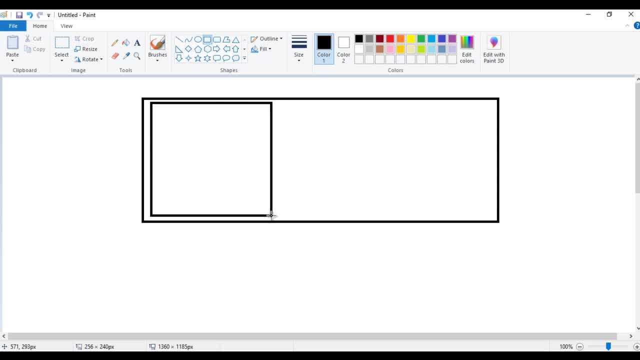 be children's. so children dues are going to be placed one beside another, right. so what you do? for the child dues you use float property and for the parent due you use the clear fix class. so very simple. we are going to understand how to place divs one beside another. we are going to 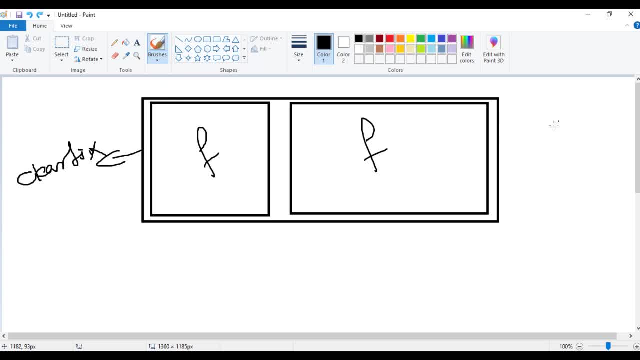 create one parent due. okay, remember that we create a parent due inside the parent due. we are going to create two child divs. okay, on the child divs, we are going to use the float property. on the parent due, we are going to use the clear property, guys. so let's create this. what i am going to do is i: 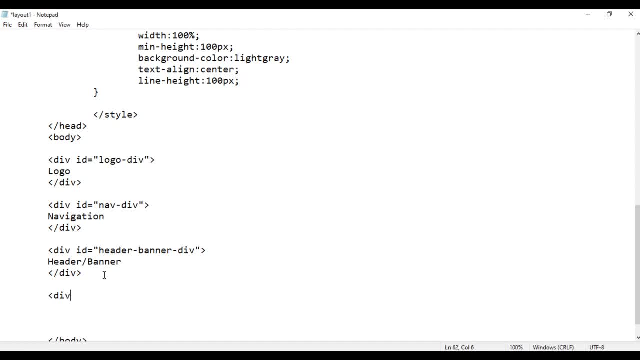 am going to create one parent to do here. so i say opening due and closing due okay, so this do. i am going to give an idea of let's say: main do, okay, that's a parent do. inside that we are going to create two child dues. so opening do and closing do, right, we have two. 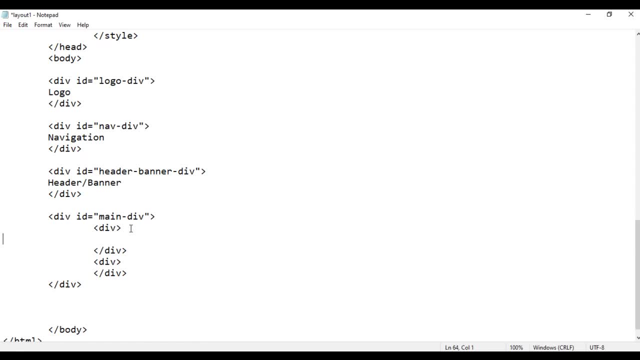 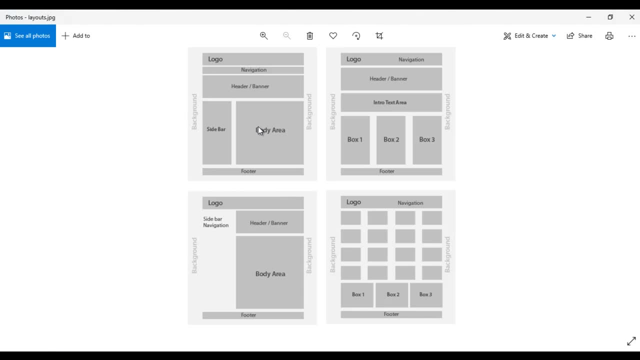 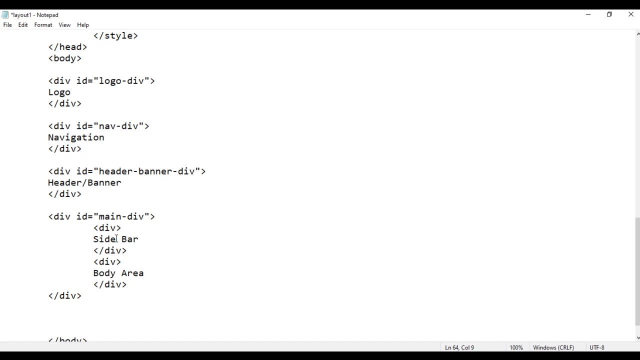 child dues. here you can see: in this do we are going to display the text sidebar. in this do we are going to display the text, what we display, body area. okay, let's say b o, d, y body area. next, let's identify them uniquely by giving an id id of s i d sidebar dash do and. to this i give. 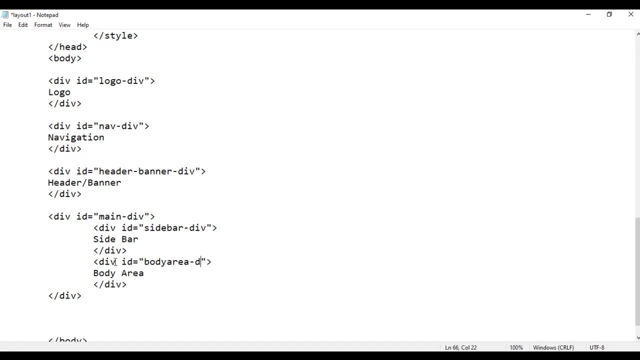 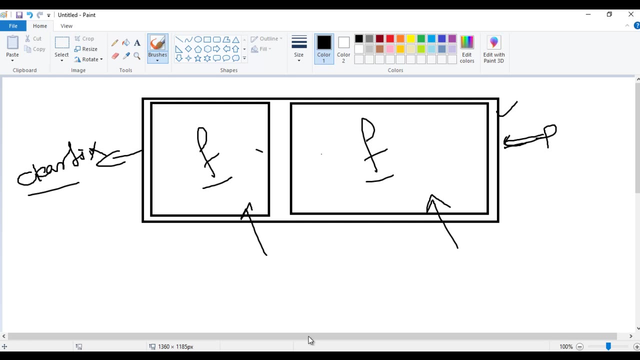 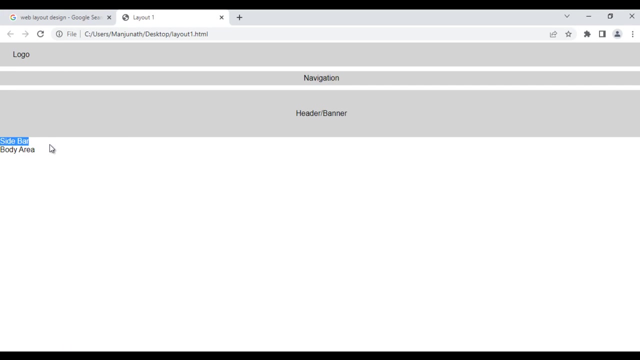 an id of body area: dash do: okay, that's our html code, guys. parent do inside that: two: child reduce: okay, that's what we have planned right. parent do two child use: okay, after writing the html, i say file save, go to browser and refresh. you can see sidebar and body area are getting displayed. 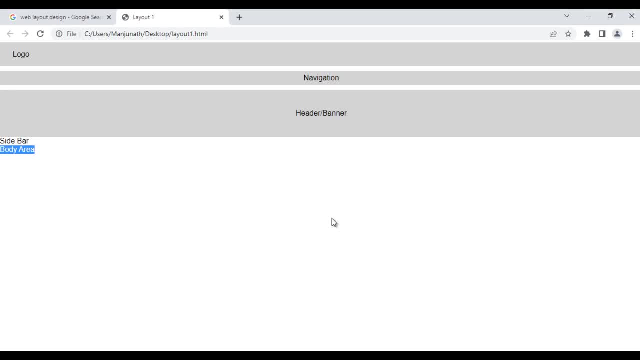 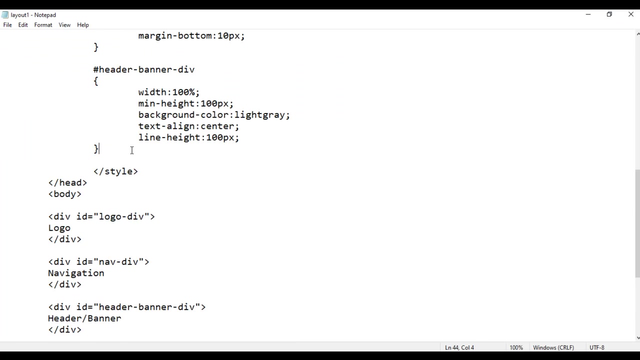 one below another. why? because divs are block level tags. they always get display one below another. we have to make them sit one beside another, guys, that's our task. okay, let's apply the styles step by step. first, let's apply the style to main: do so. here i say hash, main, do should. have the room menu and the game name, the environment we are justслиing to rank and fill. this is how we are going to: two, two, three, four and including as a list. i'm also going to apply this one to the peak. so so, starting number one, i will actually enter two, two, three, four, n, as i said, so you can have. 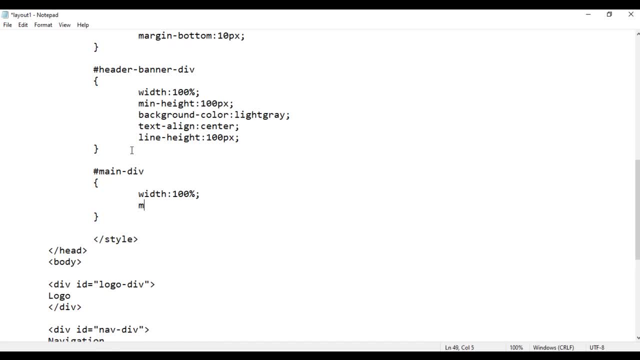 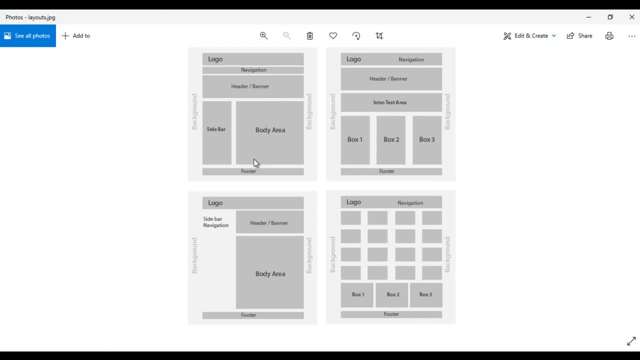 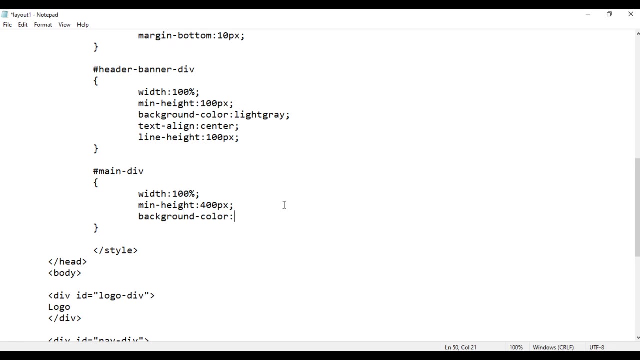 all you can work from this, such as you cute, you type n you do, because i've written this. if you don't, though, of it: width of 100 percent and then minimum dash height of 400 pixels. you see we have more height here, right? so 400 pixels i am setting, and then b, a, c, k, g, r, y, background dash color. 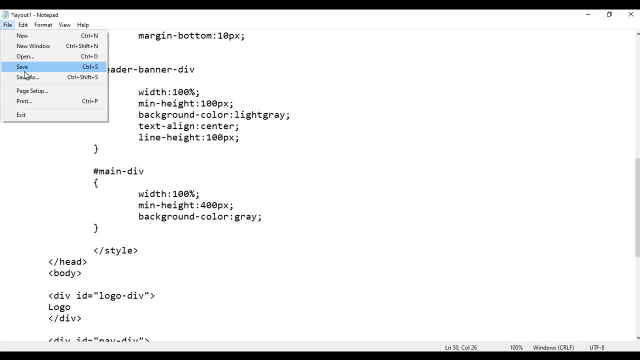 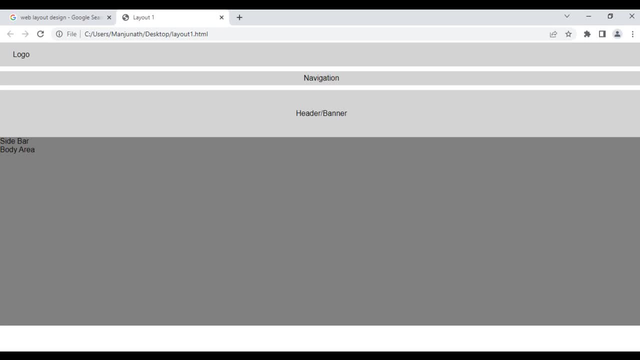 of gray. i say file save. go to browser and refresh. so we have our main view which has the width of 100 percent, height of 400 pixels, background color: gray and we need some gap here at the top. okay, let's add the margin bottom to header banner div. so we go to header. 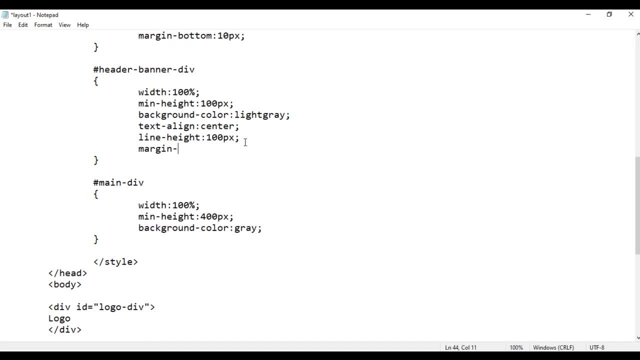 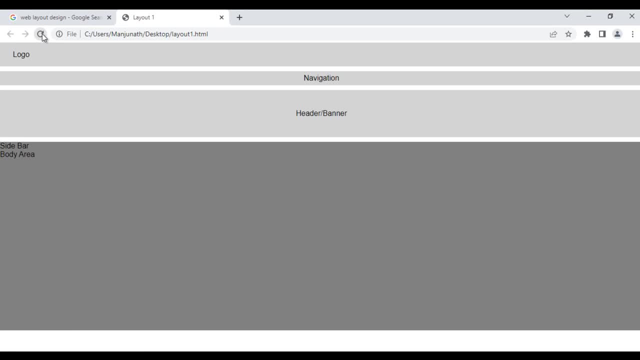 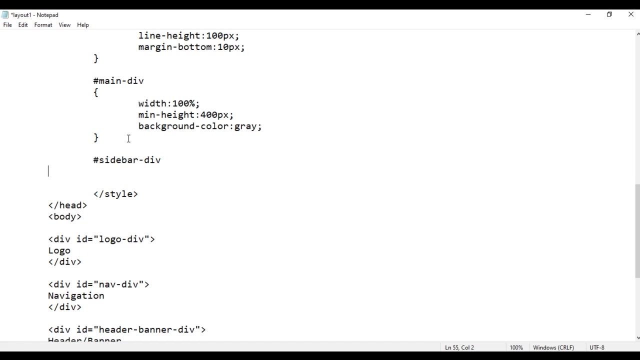 banner div and say here margin-bottom of 10 pixels. if i say file save, go to browser and refresh, we got the space, awesome. next we are going to apply styles to sidebar div and body area div. okay, so i come here and say hash, sidebar dash div should have. should have width of. 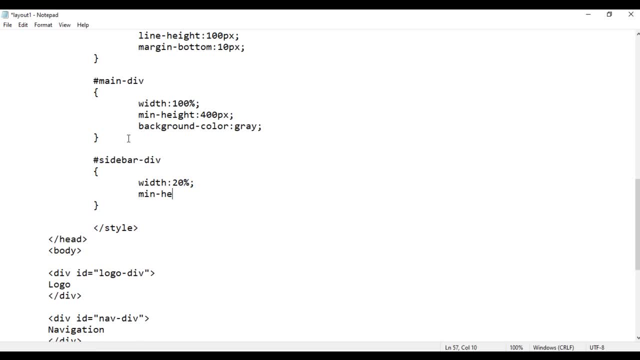 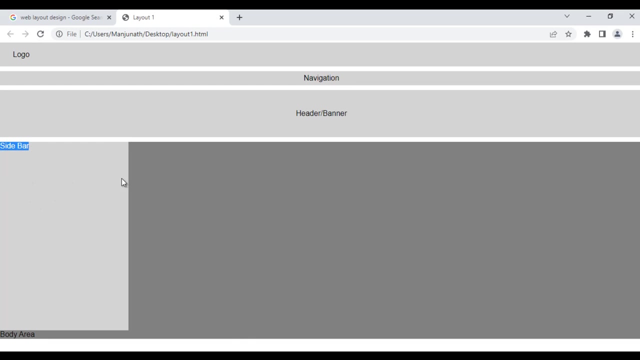 let's say 20 percent minimum dash height of 400 pixels, right, minimum height of 400 pixels. and i say here background dash color of light gray. so if i say file save, go to browser and refresh. you see, our sidebar has width of 20 percent. 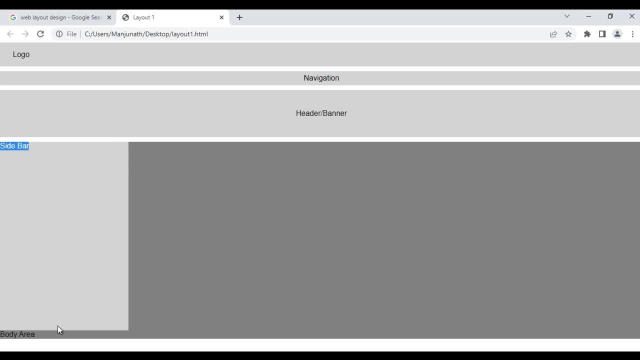 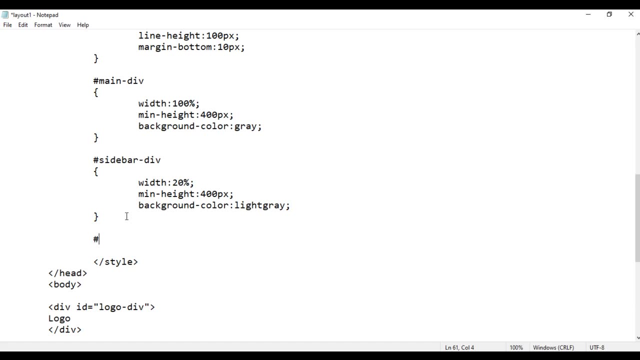 height of 400 pixels. background color: light gray. here we have the body area- right body area div, which is below: let's apply the style to that also. so what i do here hash body area dash div. opening flower bracket, closing flower bracket. width. i am going to set, let's say, 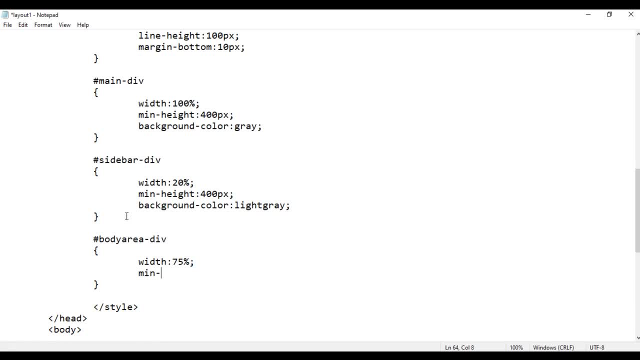 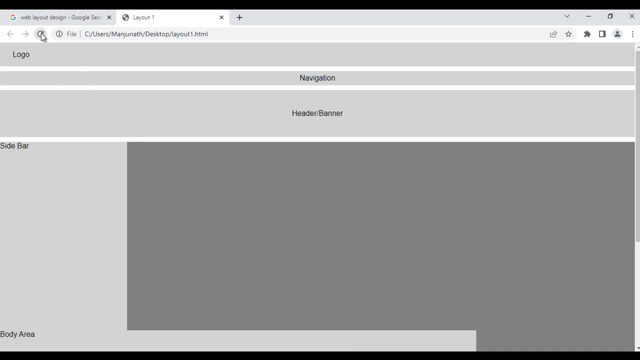 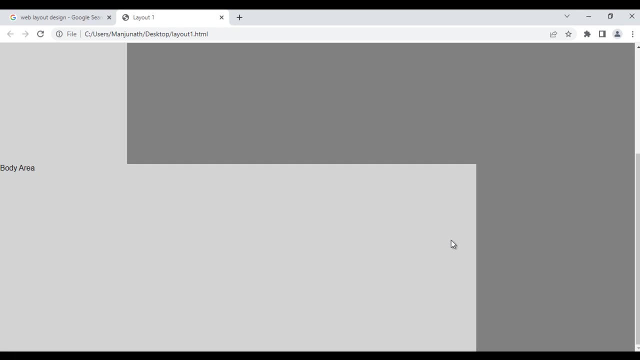 75 percent and minimum dash height of 400 pixels and then background dash color of ligst, light gray semicolon. i say file save, go to browser and refresh. you can see that we have body area which is of 75 percent width. right, so we have sidebar above body area, below what we want. we want to place them one. 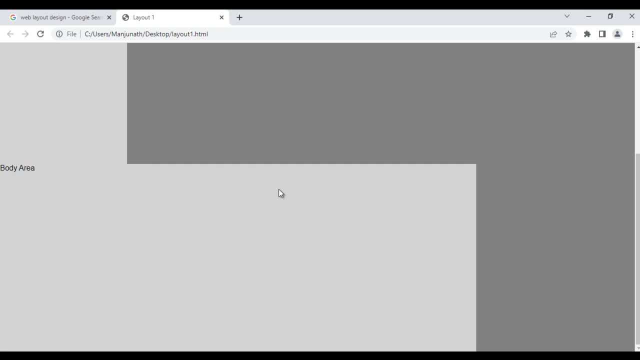 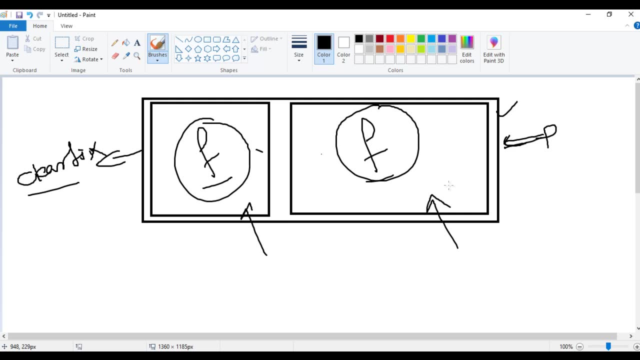 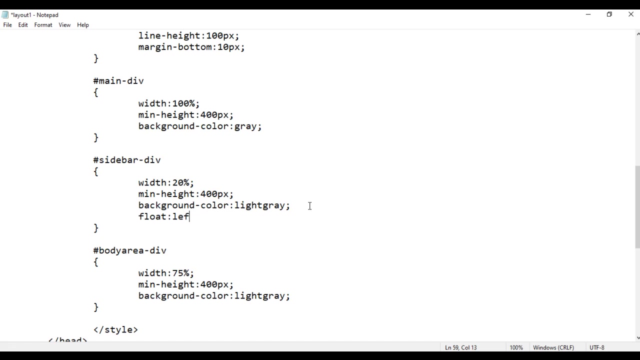 beside another. so i told you how do you place them one beside another. so i told you how do you place the elements one beside another- child elements: if you want to place one beside another, you have to use the float property on both of them. so i come here. sidebar div should float to the left side. 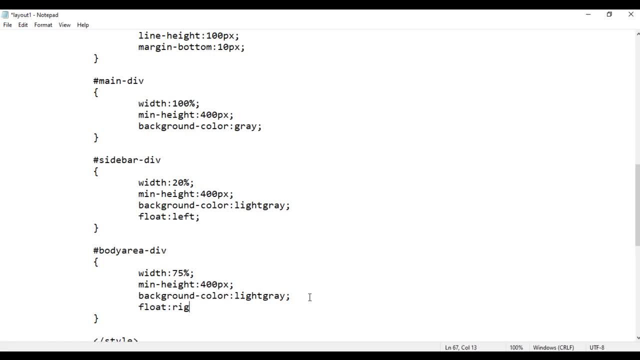 and body area div should float to the right side and we are going to remove the minimum height value from here, okay, so when i remove the minimum height, okay, what happens? as both the elements are going to float right, they are going to float, one floats to the left one. 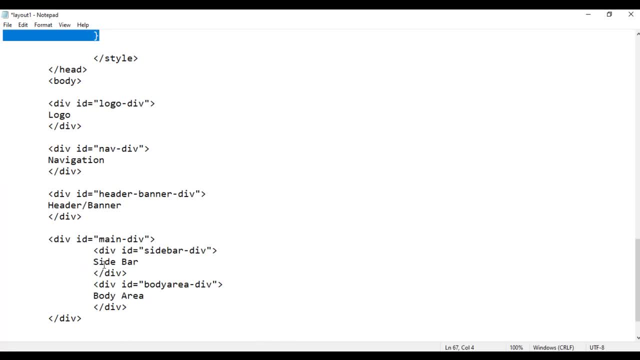 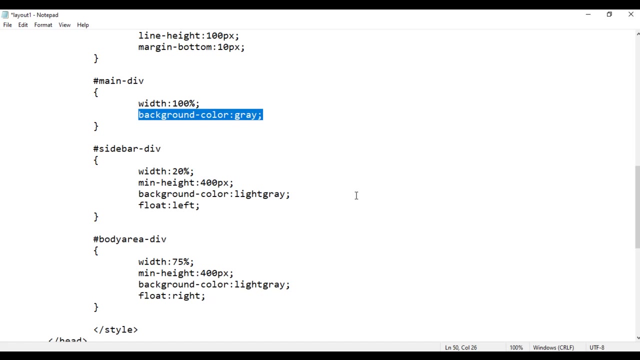 float to the right browser. considers there is no element inside the main div. there is no element inside the main div, so main div is not going to have any height. if there is no height, definitely you don't see the background color gray displayed there. if there is no content in the div, what? 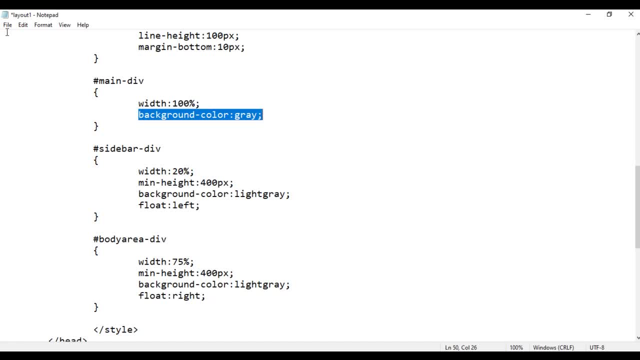 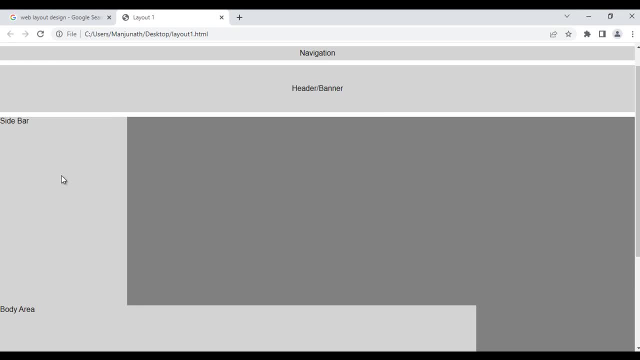 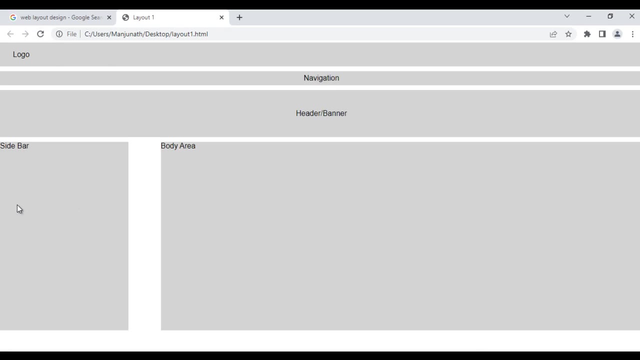 happens. it is not going to have any height right. so check out what happens. if i say file, go to browser. if i say refresh, sidebar and body area are going to sit one beside another. we don't see this background color gray. if i say refresh, you see, sidebar is on the left side. 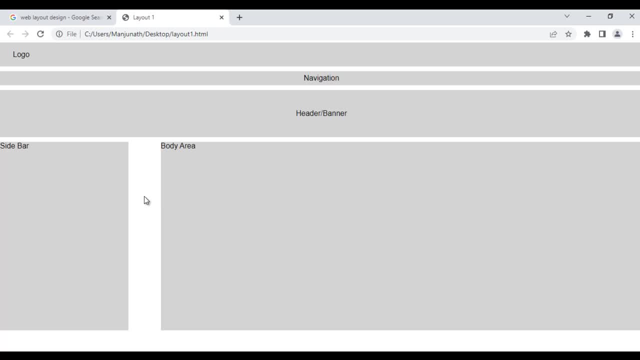 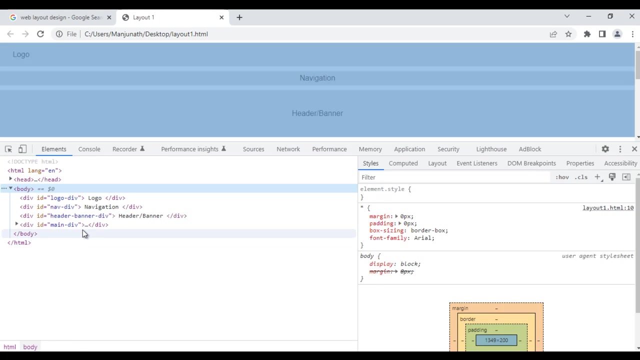 body area is on the right side. we are not having here that gray background. we are not having the main div available here. why? because main div height is set to zero. now you can observe clearly if i go here more tools and developer tools. if you see the main div right. the main div has zero pixel height, right in this place. you observe. 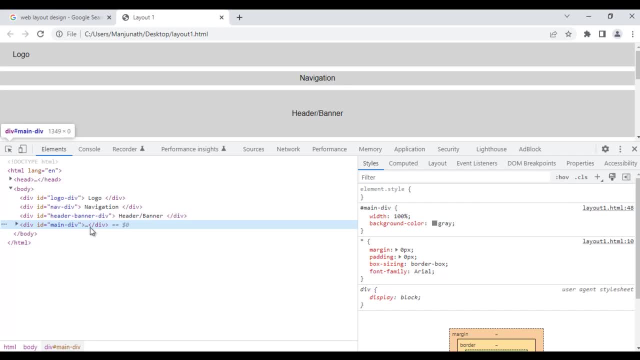 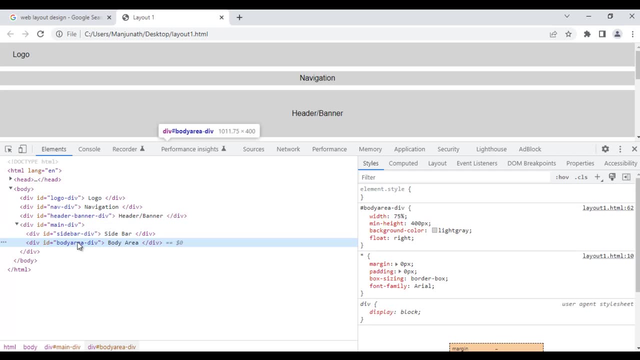 the main div has 1349 pixel width but height is zero pixel. why? because in the main div, whatever the elements we have- sidebar div and body area do- they are floated. when the elements float, okay, then browser considers there is no content inside that parent div. right, both the elements. 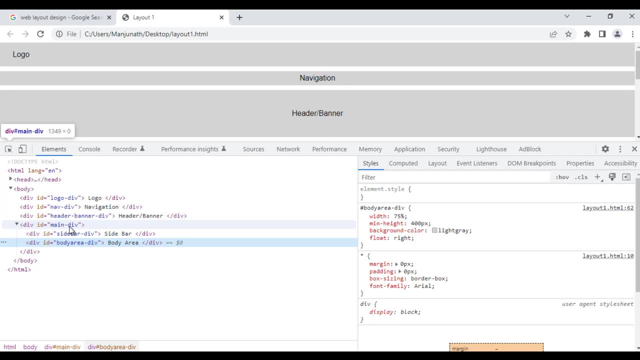 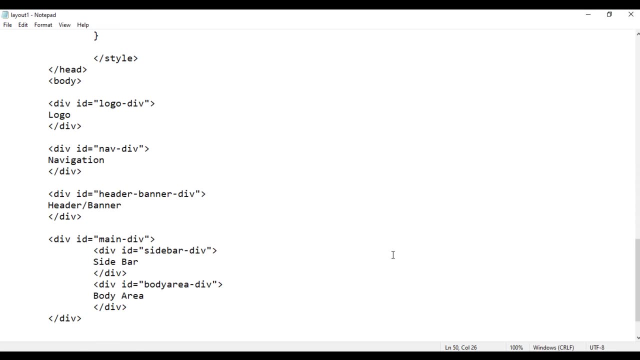 are floated, there is no content in the main div but there is no content inside that parent div. when there is no content in the div, definitely its height will be zero. so we have to bring that height back. to bring the height back, we are going to use the clear fix class. so what are we going? 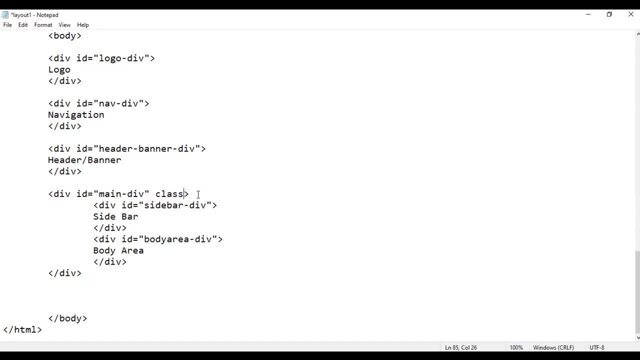 to do to this parent, do? we are going to use a class called as clear fix, okay, and let's apply the styles. so here i say: dot, clear fix, colon, colon. after opening floor, back at closing floor bracket. so what are we telling? select the html element which has the class attribute value set. 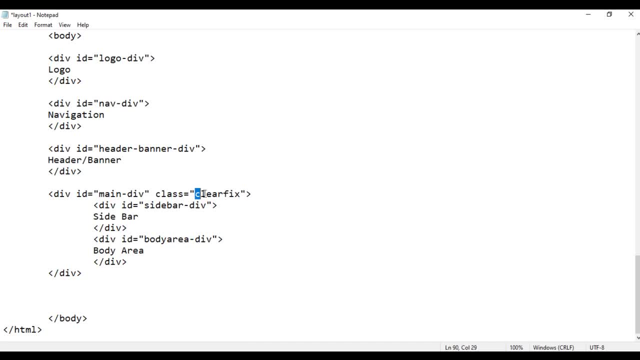 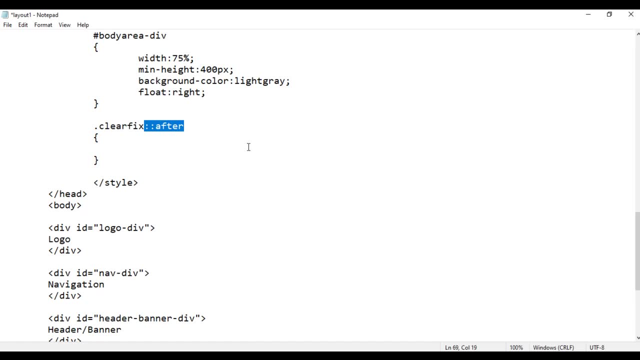 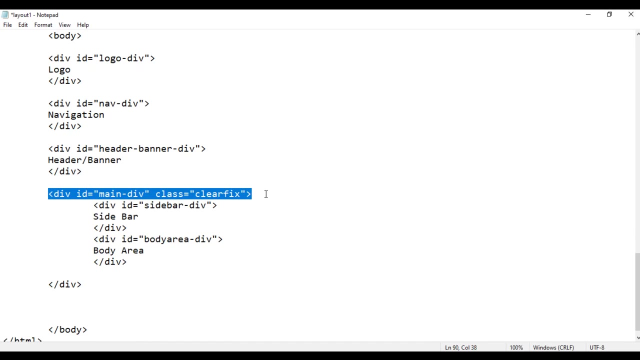 to clear fix. okay, this parent div has the class attribute value set to clear fix colon. colon after is a pseudo element. what it indicates, it indicates after the content of it. after the content means somewhere here. so these two divs are the content of this main div. so after the content we want to. 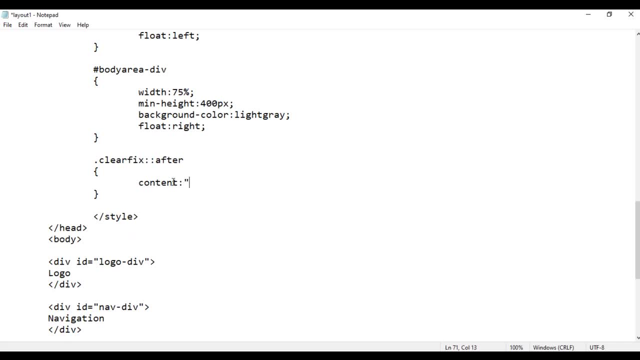 generate this content. what we want to generate content should be: space should be generated. its display should be set to block and clear both. we don't want to have any float effect- float left, float right. we don't want to have any float effect on the parent. so clear both. i told 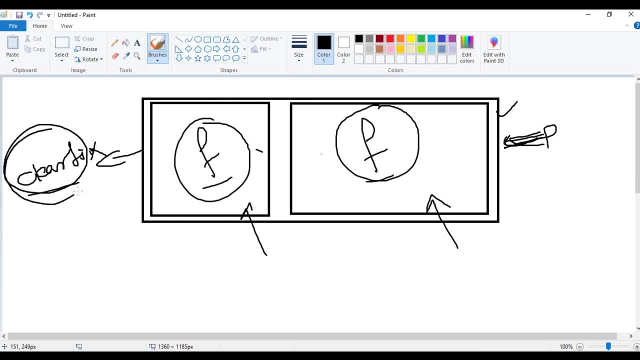 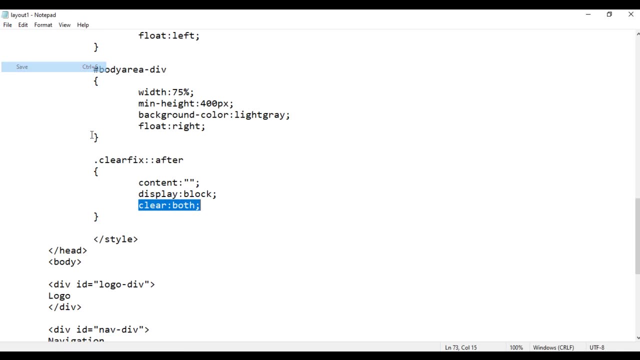 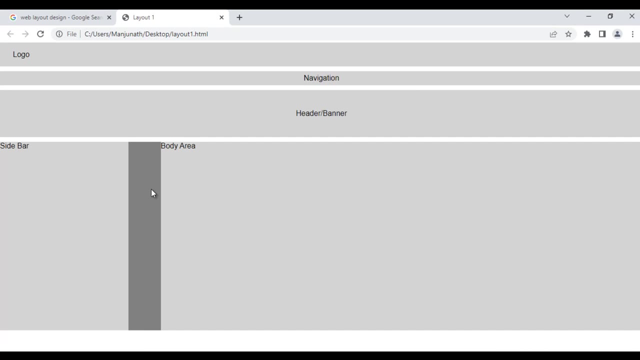 you right on the parent. you have to use the clear property. right float property you will be using on the children or the child elements, and clear property you will be using on the parent. very simple right now. if i say file save, go to browser and and refresh. you see we got the height back. we. 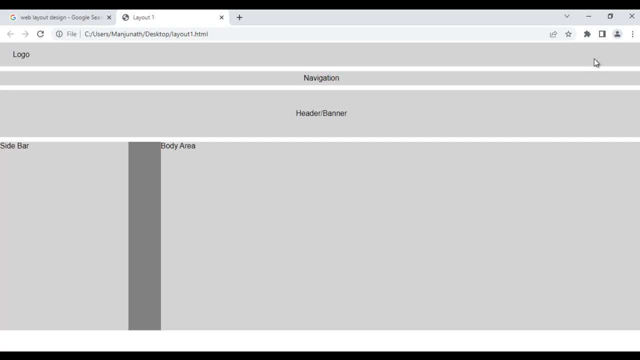 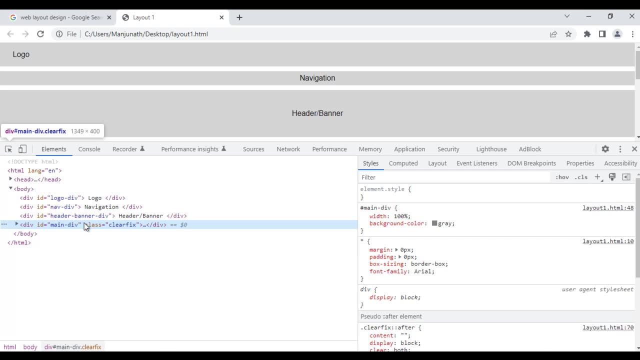 got the height back to main view. we are seeing the background color gray here. if i go here- more tools and developer tools- and if i click on the main view, you can see now it has 400 pixels height. can you see? the main view has width of 1349 pixel width and height of 400 pixels. so we 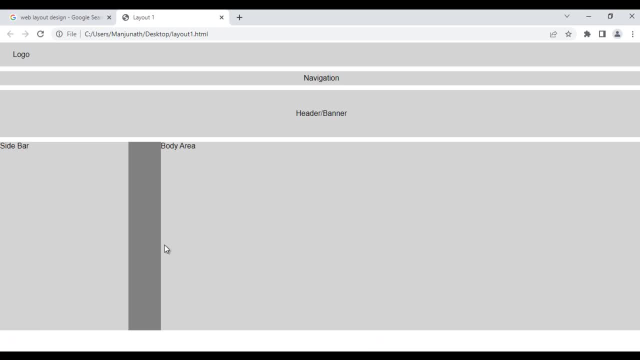 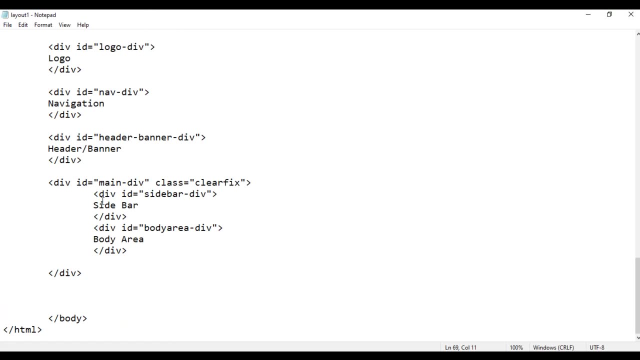 got the height, guys. so that is how you will be using the clear fix property, which is very, very useful, guys. clear fix class. so this is how you will be placing the divs one beside another, float the inner elements and clear fix the parent. very simple, guys, right. 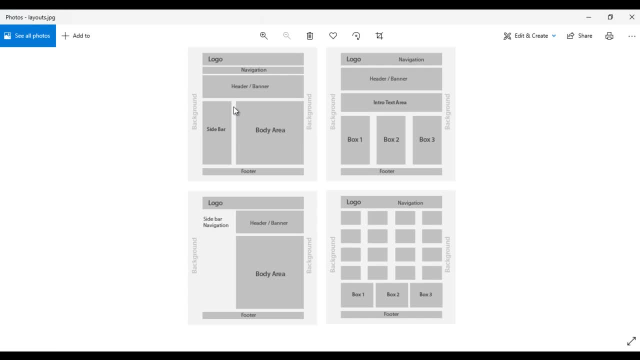 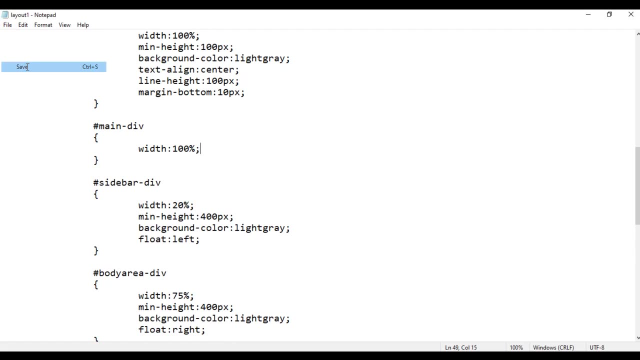 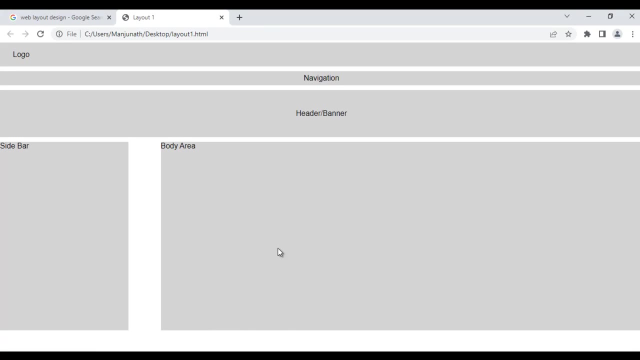 we are able to do that. next what we want: we are going to remove this gray color background. so simply we remove the background color gray from the main view file. save, go to browser and refresh. ok, done. let's see what we have to do next. next we have to place the sidebar and body area. 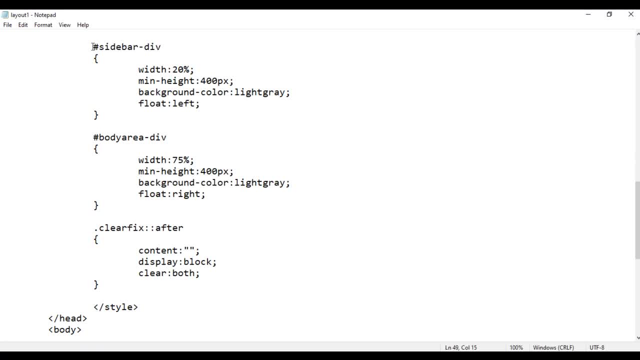 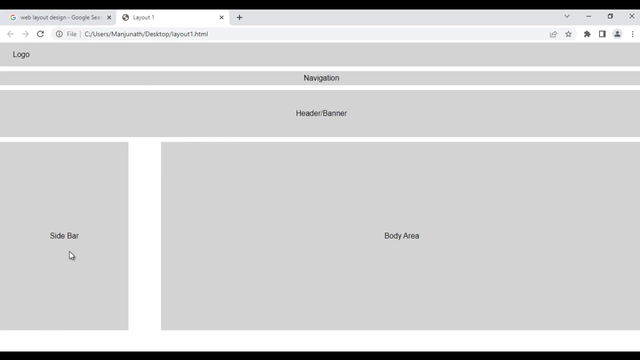 horizontally and vertically center. very simple, it is very simple, right? so go to sidebar div and say here: text dash align center. then line dash height should be 400 pixels, same as the minimum height. copy this code and use that in the body area, save it, go to browser and refresh. you see they are placed center. good, what is left? we left with. 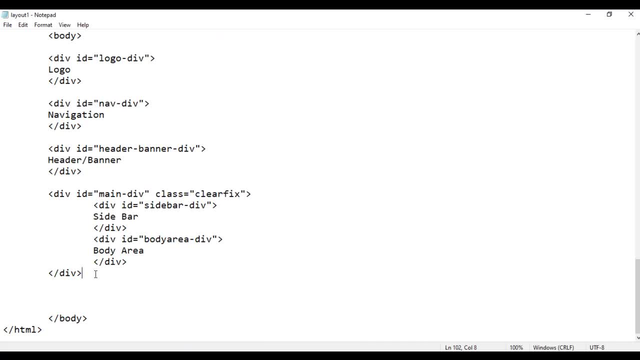 the footer div and it's very easy to create the footer div. just below this div we create another div- opening div, closing div- and the content we display footer. and i'm going to give an id of footer dash do. and then i come here and say hash. 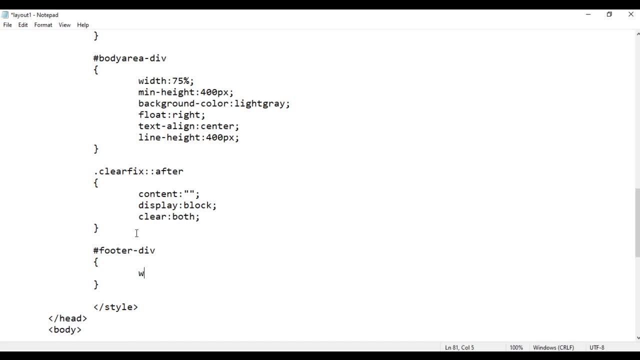 zero, less than measure, and k one, two, two, three here. so if you are using now Nordic Alaska, next for the footer div. by now you are looking atlish sentido. i give slash and try to compare here that the footer will be there. it is there, but i am going to manually. 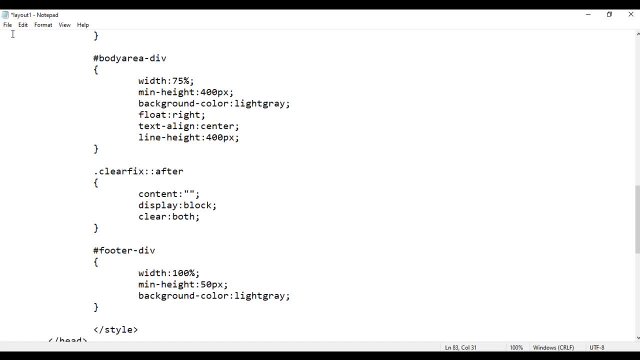 keep the footeresis integer very tiny so that, if you see, if we define weight, then the footer div should have width of 100 percent and then he igsd height of, let's say, minimum, a minimum-height of 50 pixels. background dash colour should be light gray. i am going to save file. save. go to browser and refresh. see, we got the footer div p, But there is no space above the footer div. so what? NO space above the footer div? so what will table as a footer div? is it can sentiment? 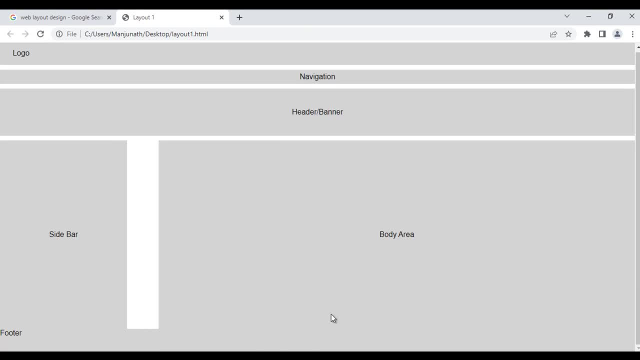 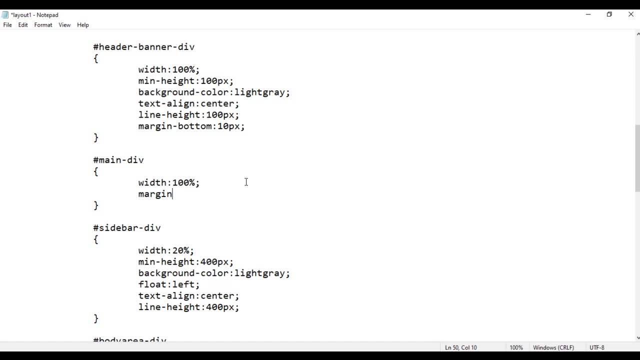 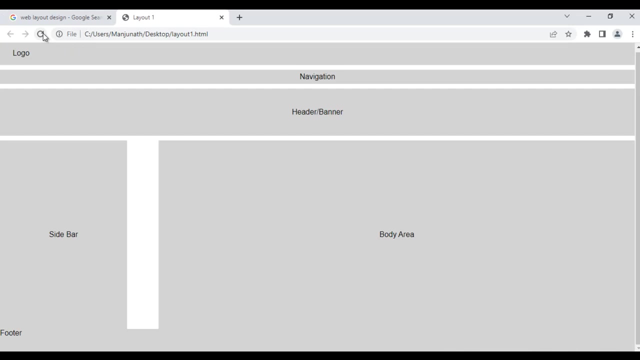 file save, go to browser and refresh. see, we got the footer div. but there is no space above the footer div we can do. We can go to the main div and say here, margin-bottom of 10 pixels. I say file save, go to browser and refresh. See, we got the space. Let's place the footer horizontally. 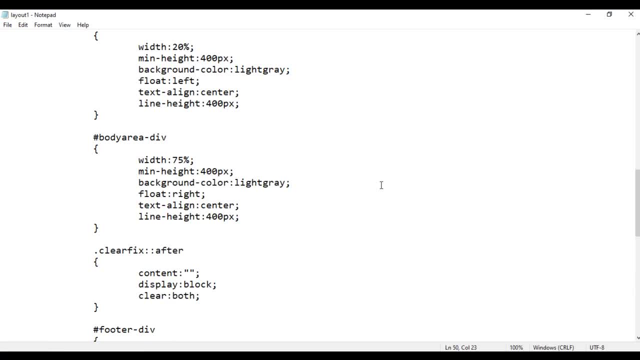 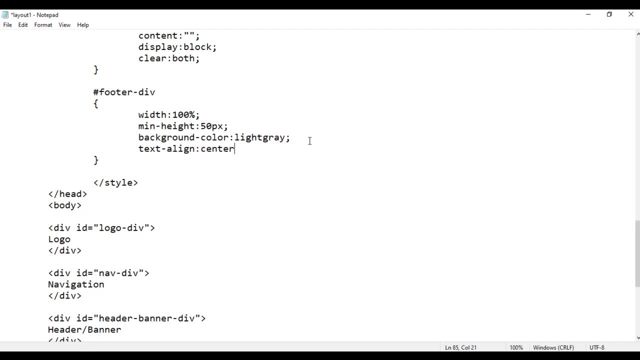 center, vertically center, footer text, right. So for that, what we do, You already know, simply you use here text dash, align center and then line dash. height of 50 pixels, Same as the minimum height File. save. go to browser and refresh. See, we place the footer text. 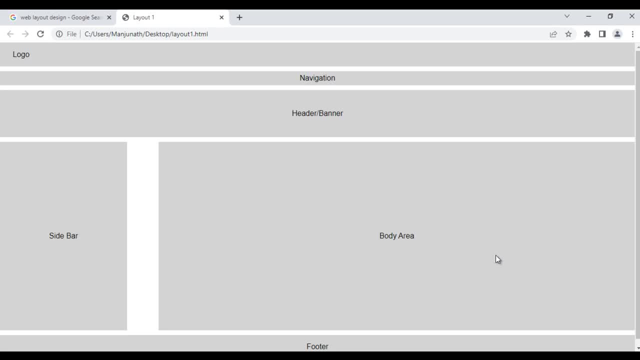 horizontally, vertically, center. Now here our divs. this layout is actually fully stretched right, It is fully stretched. What if you want the layout should be center aligned? Okay, But we want it to be something like this: on the left side, We want to have some space. 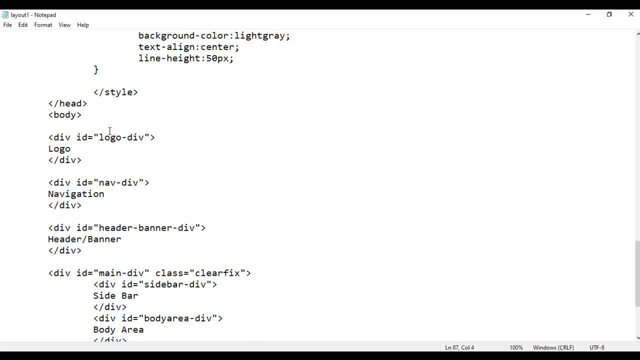 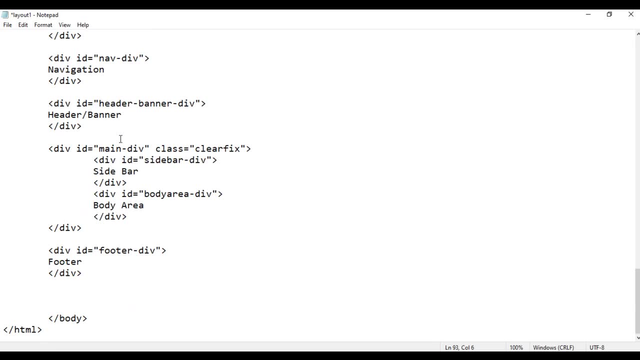 right side. We want to have some space. So for that, what you do, you put all this content inside another div. So we make another div here, opening div and closing div. So this div is going to work like a wrapper. So ID I give here wrapper dash div. So this div. 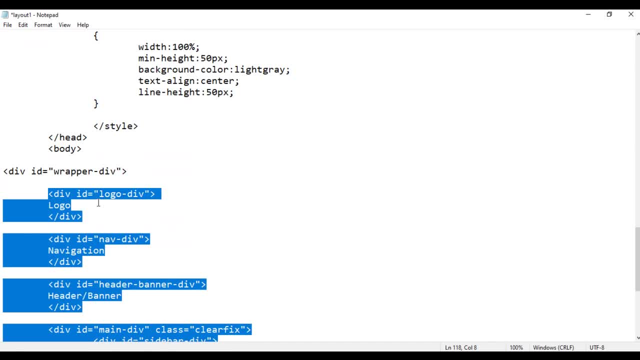 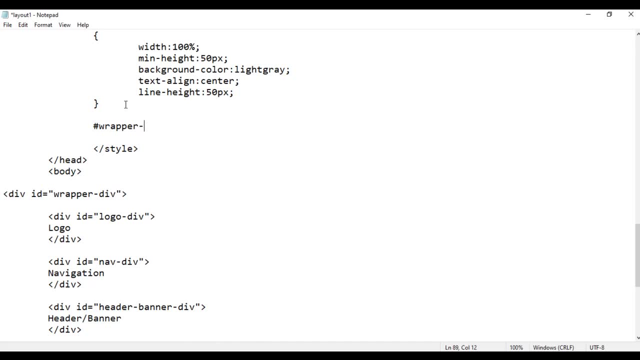 is going to wrap all this content. Okay, So we're going to wrap. We're going to wrap. apply the style to wrapper div. So very simple. I say hash, WRAWPR, dash div. Wrapper div should have width of 100%. Okay, We are not going to set any minimum height here, We are just 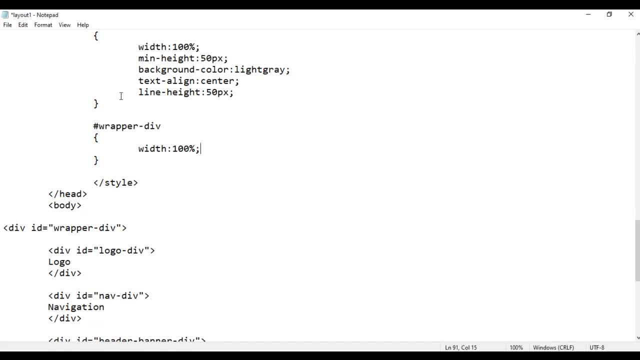 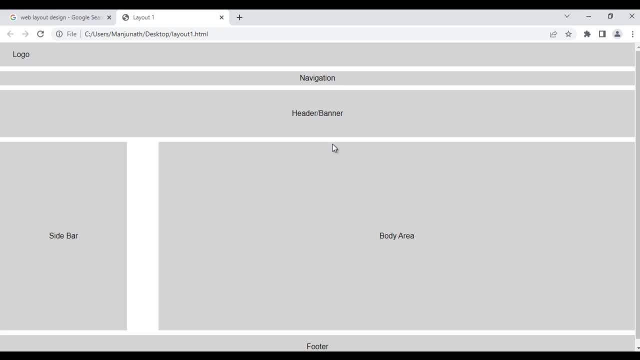 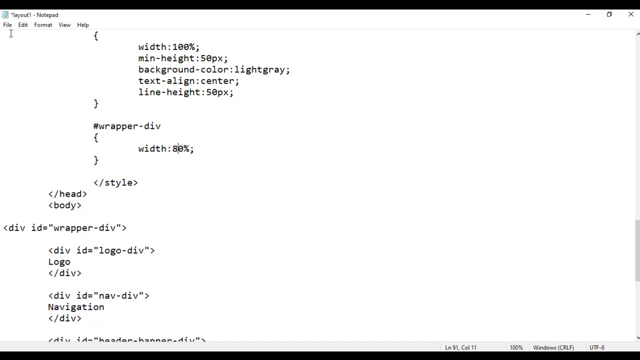 setting the width of 100%. Okay, So if I just save it, combine, refresh, you don't find any difference Because wrapper div has 100% width. all the elements are going to be 100%, No issues. But if I set it 80%, file save, go to browser and refresh. You see our wrapper. 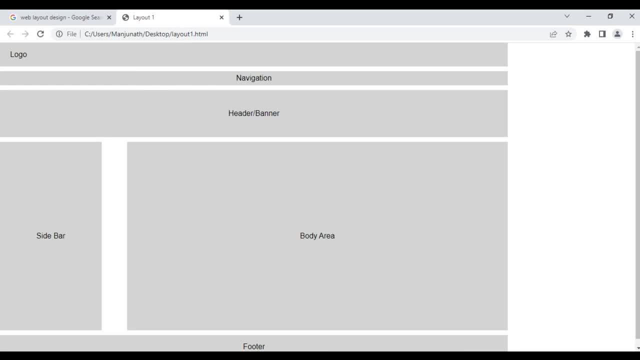 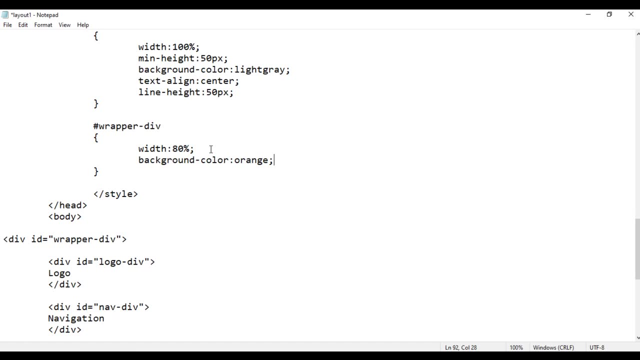 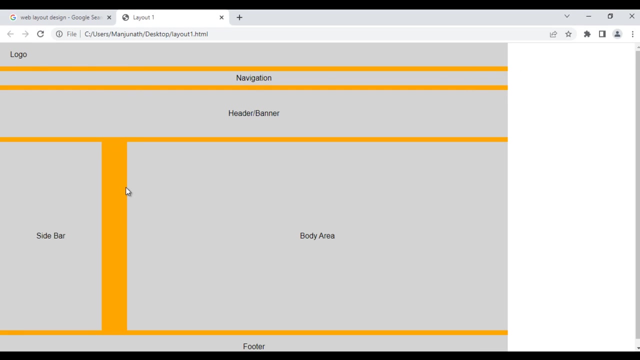 div has 80% width. Let me set the background color to show you what is happening. If I say here background dash color of orange, I say file save, go to browser and refresh. So this orange color box indicates the wrapper div guys. So wrapper div has width of 80% and 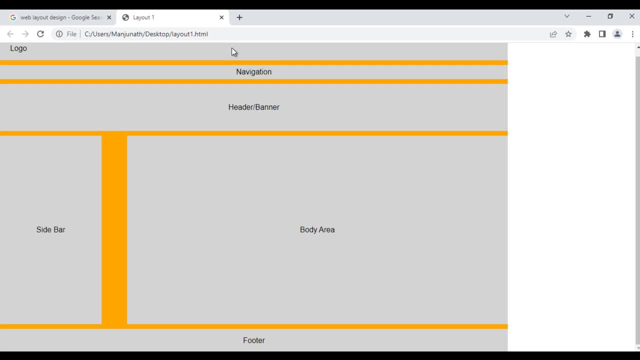 the inner elements. we have set the width of 100%, So always remember the inner elements are sized with respect to the parent, So inner elements are having 100% means they are 100% with respect to the parent width. So parent is 80%, So these are also 80%. Very simple. 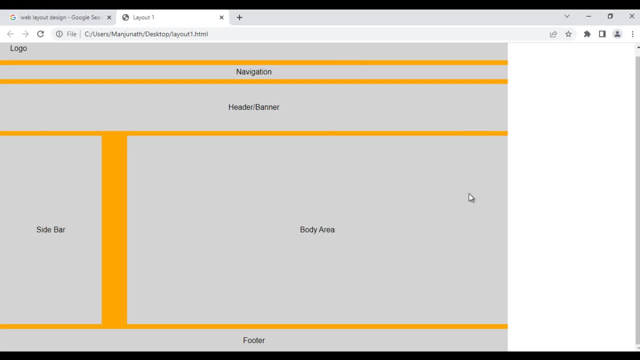 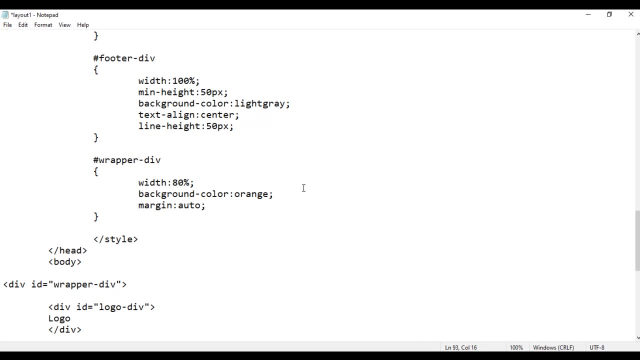 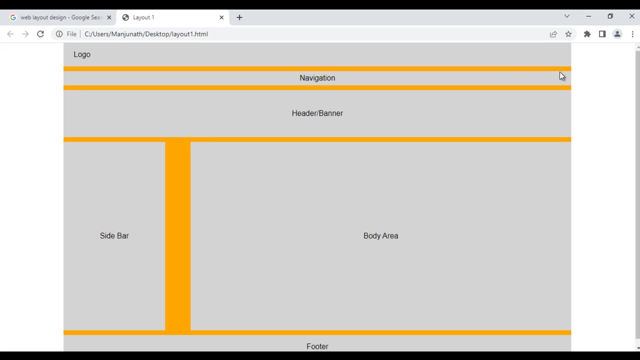 Okay, Now let's play this entire thing: center aligned, Center Aligned. so for center aligning, we just simply say margin auto. when i say margin auto to wrapper, do file save, go to browser and refresh. you see the content is center aligned. everything right, left, side, right. 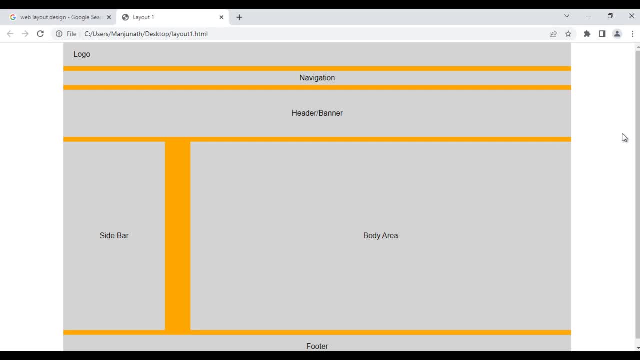 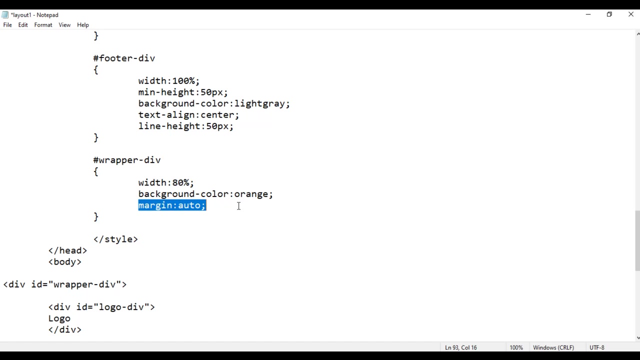 side, we automatically got some margin. if you wanted to make it 100, it's very simple. just come here and say 100 file, save, go to browser and refresh fully stretched. you want center aligned? simply say here 80. we have margin auto. so no problem. save, go to browser and refresh, see. 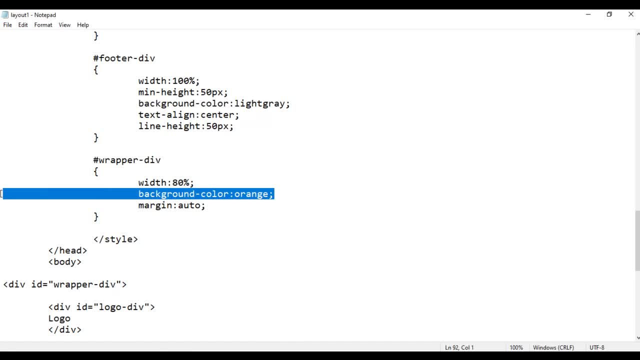 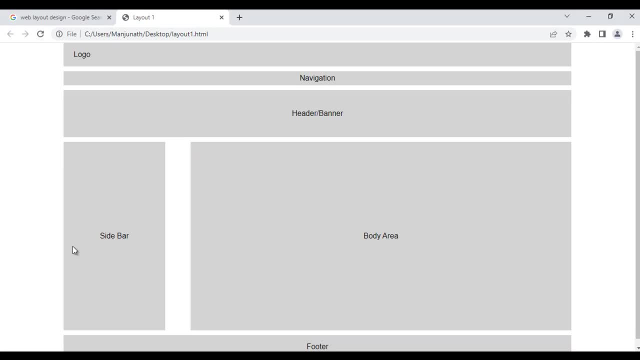 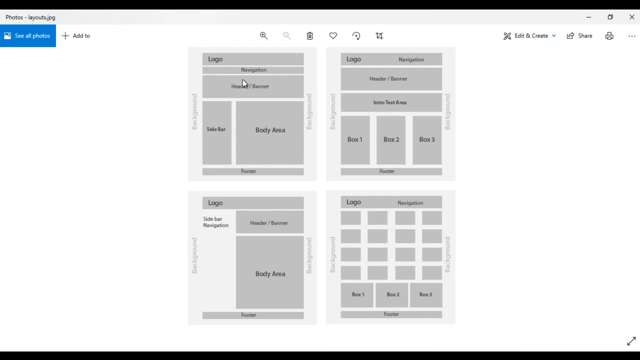 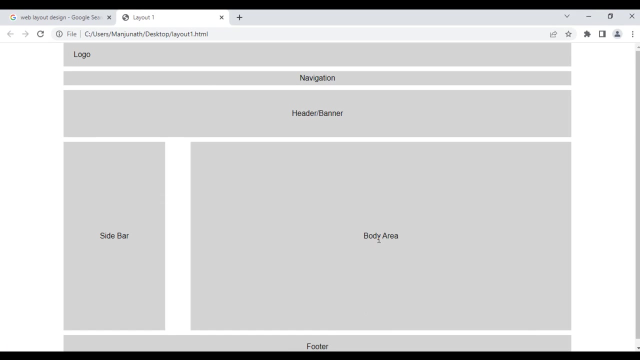 and now i am going to remove this background color orange from the wrapper. do file save, go to browser and refresh. you can see that we are successfully able to create the first layout. that is the layout one. right, guys? congratulations guys. i suggest you people to watch this video again and again. okay, understand everything clearly, try this yourself. if you try it. 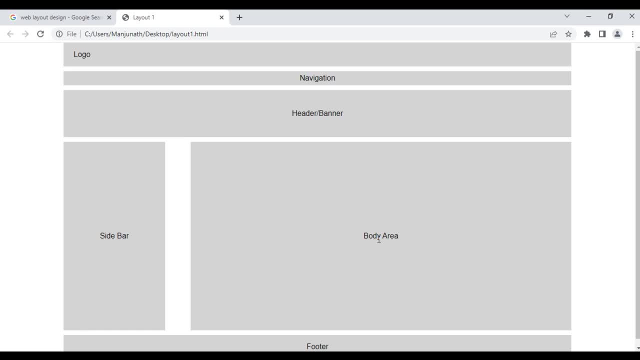 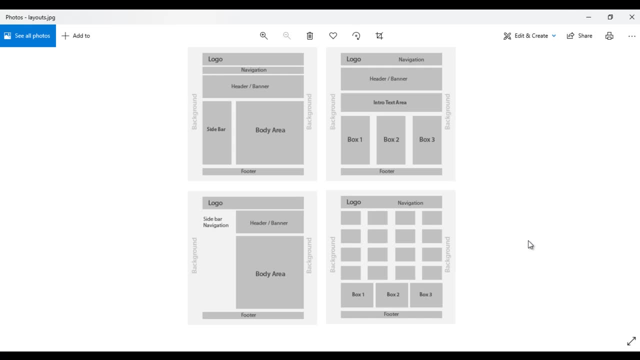 yourself, you get more clear idea. guys, in the upcoming video tutorials we are going to understand the next layouts one by one. okay, once we create all the layouts, you will be able to create any layouts. you will be able to create any layouts. you will be able to create any layouts. you will be